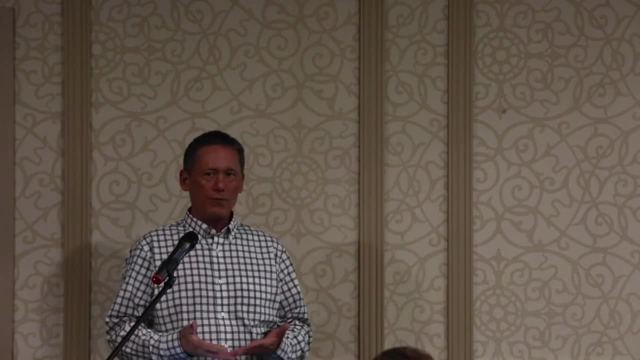 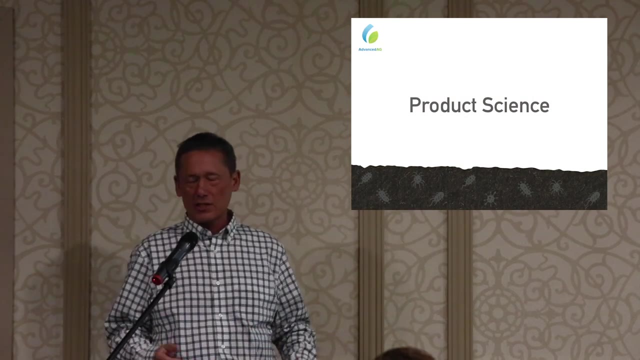 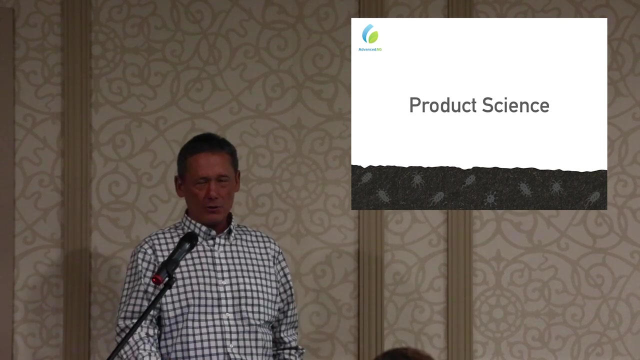 or adding fungi, to adding useful functions into the soil, And it's really the theme. And if there's anything to take from this product science presentation, it's: what functions can we add into our soil to make it healthy for the crops and to promote the biodiversity of the whole? 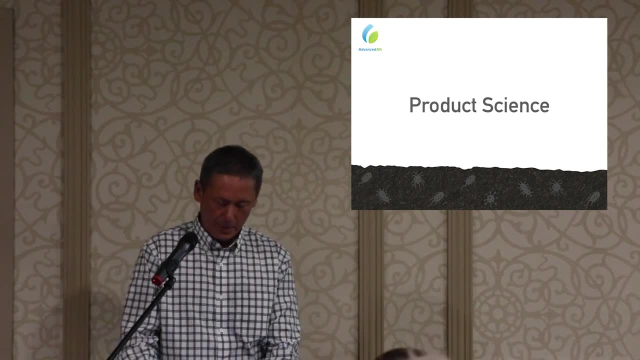 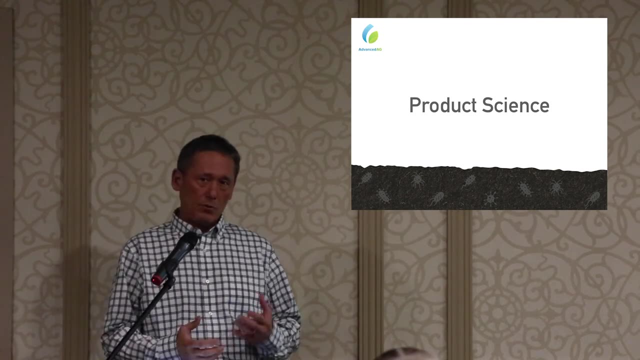 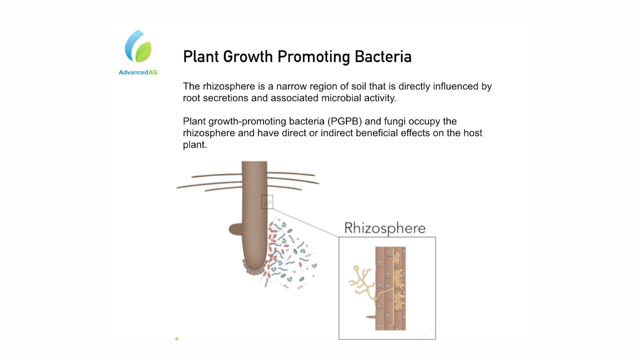 system there. So as we go into that, of course we're going to start talking about the rhizosphere, which is that little narrow zone right at the root soil interface where you have plant exudations, you have bacteria, you have fungi. It's a real complicated thing. 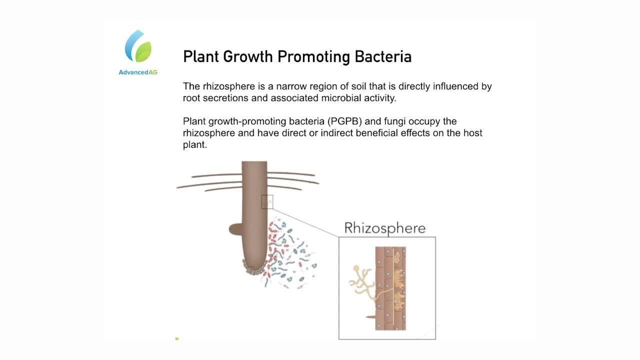 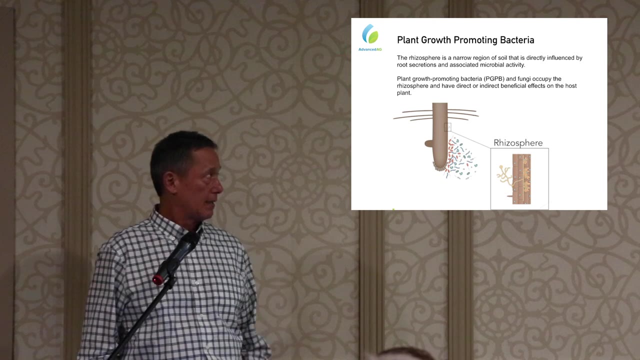 We all know and have heard the term and it's really important to have it right, but we're not sure what that means. So all kinds of researchers have been looking at plant growth promoting bacteria or plant growth promoting fungi, And I'm just going to, as we go on, just focus on plant growth promotion. But it's been going on. 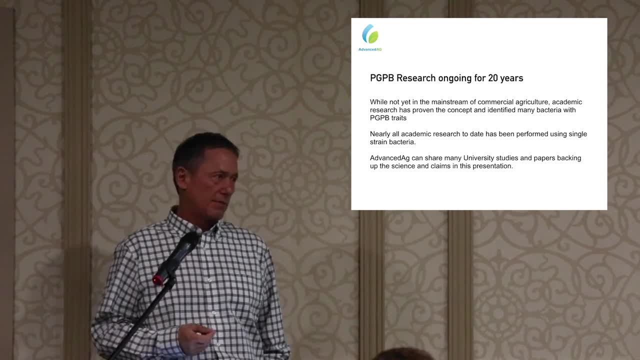 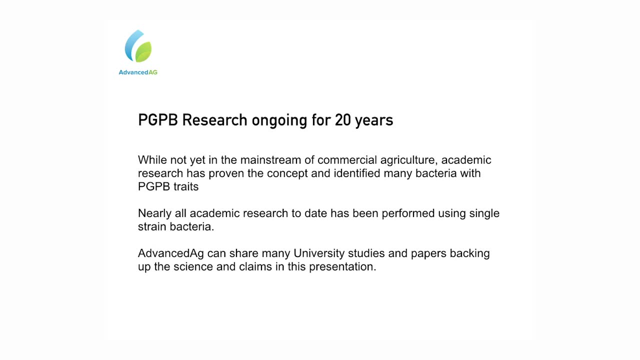 for a couple of decades now And you know, as we do in academia, sometimes you can't change 20 variables and get an answer. So a lot of times you know, and most of the research, whether it's fungal or bacterial, it's with a single species and they're looking at. you know very defined. 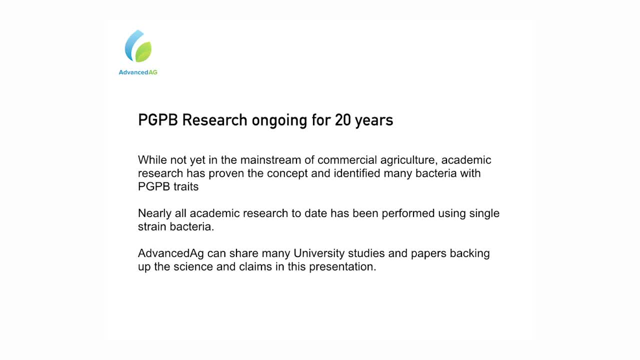 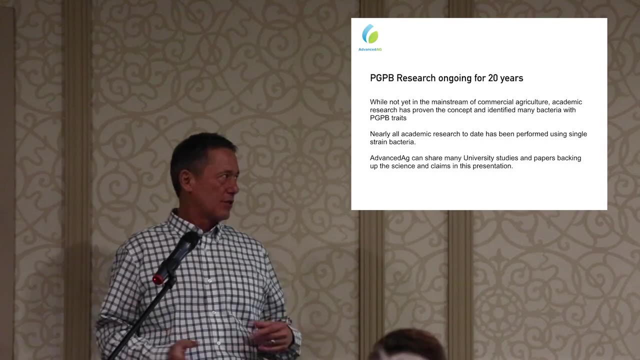 things I think it's important for us in the practical world to understand. you know how to take any aerial view of a crop field And if you see something that looks homogeneous, all the same you're not using your eyes. It's never that way, So there's so many differences. 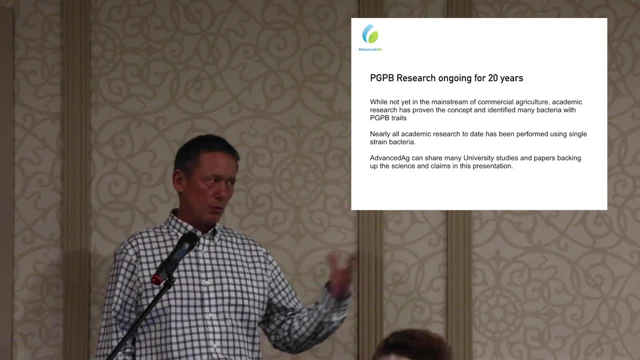 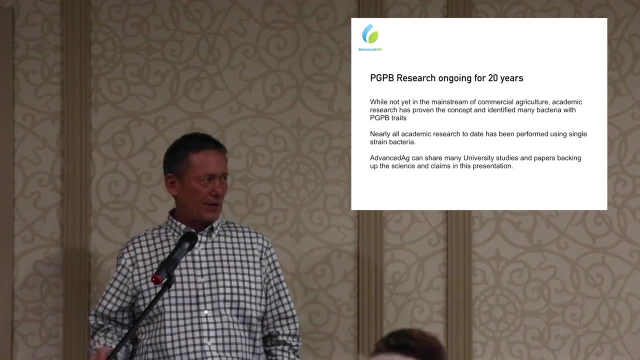 you know, even from point A to point B, within the same field, where the soil is different, the microbiology is different. So you know, a single strain going into a given field, you know, does it really pass the smell test? And I think the answer is it really does. 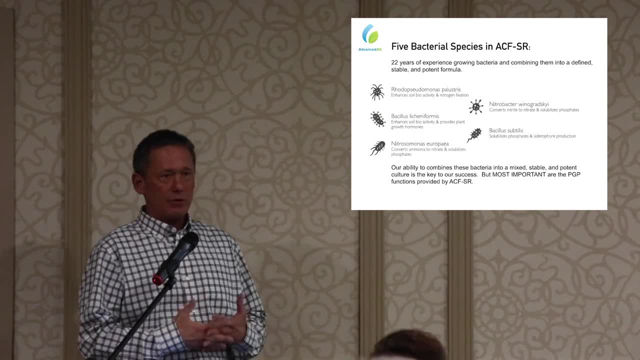 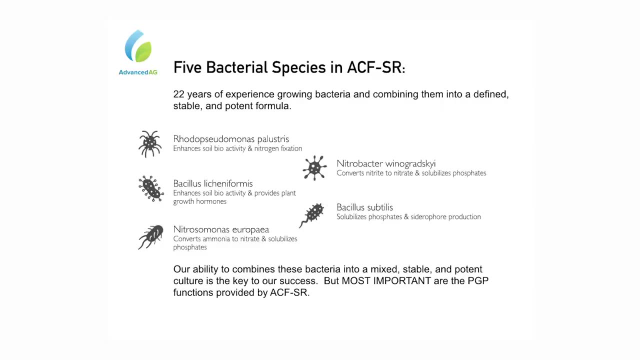 Not having said all that you know, we do disclose. just as Travis pointed out, we have these five species of bacteria in the ACF main formula For one. these are all on the Canadian DSL, the domestic substances list, where you can bring them into the country, And we have one. 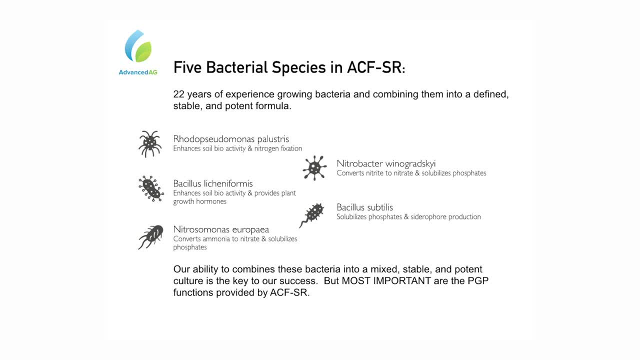 rotosudomonas. that's a photosynthetic that has ability to work with oxygen, without oxygen, with light, without light It fixes nitrogen, It fixes carbon dioxide, It breaks down all kinds of things. So it's a workhorse and it's involved in a lot of cutting edge research. It's maybe. 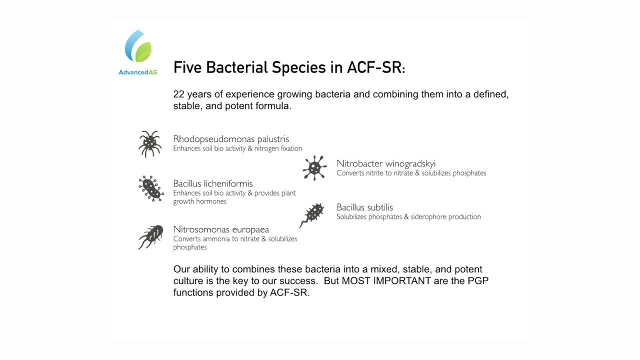 looked at something that will help with greenhouse gas emissions and turning atmospheric CO2 into something more useful. But along with that we have two bacillus species, That's, a lacaniformis and a subtilis, And we have a lot of other species And we have a lot of other species And 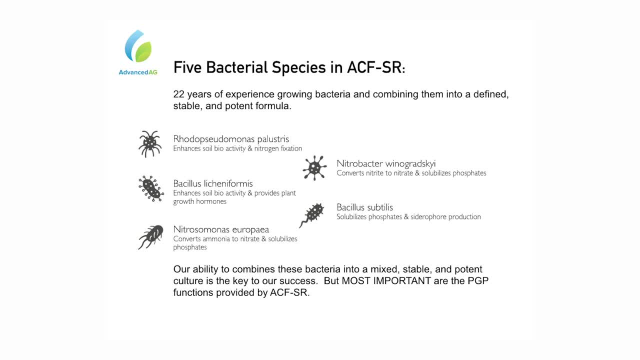 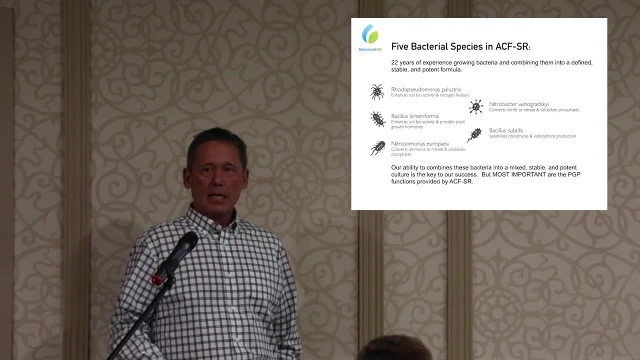 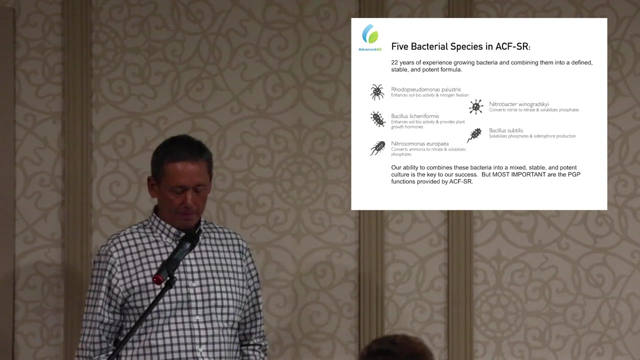 we have two nitrifying organisms. Having said all that, and you know, those are all present, identifiable and clearly cut. the species really aren't that important, which is going to sound crazy, But it really. as we go through this, you'll understand Whether it's plant growth. 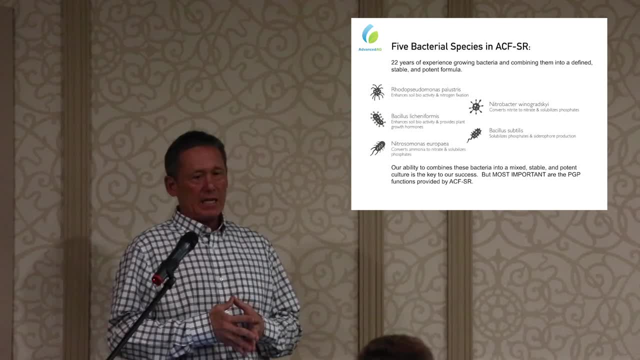 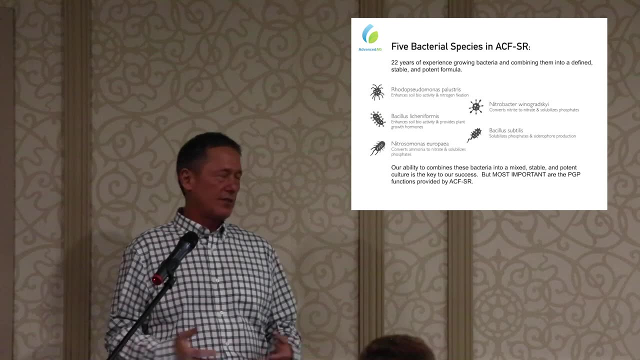 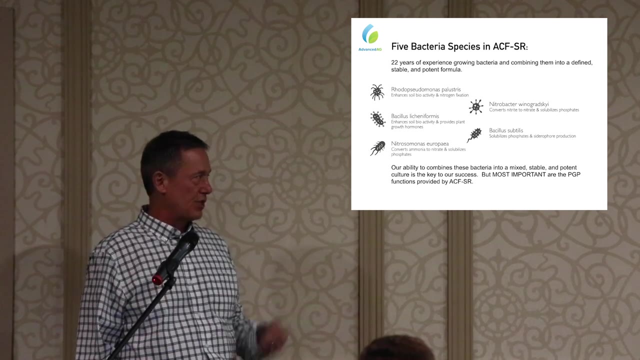 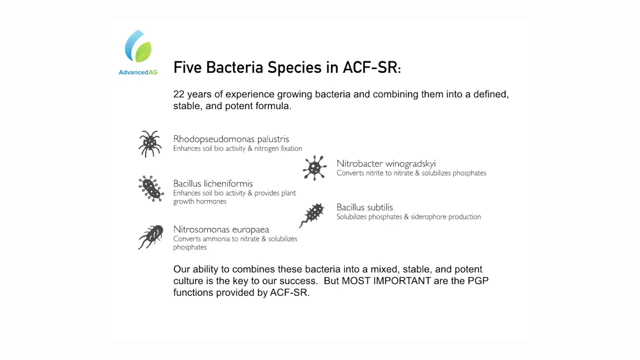 promoting bacteria or fungi and you look for any summary paper, you'll find that there are several recognized, obvious and very important species, And so you know we have two nitrifying organisms that are in different ways that the microbes can help the plants. 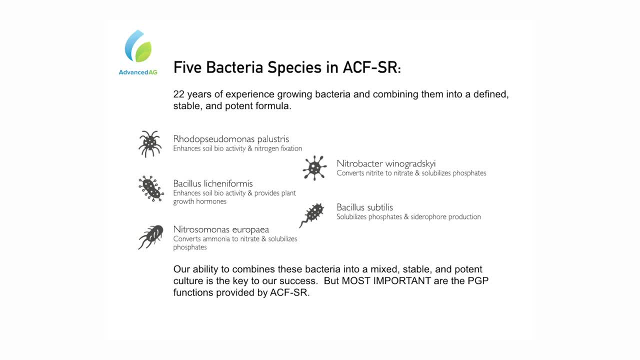 And for direct plant growth we have nitrogen fixation, pulling nitrogen out of the atmosphere and making it into an organic form that the plant can use. Phosphorus solubilization- very important. We' will talk about that along a similar self line of potassium hold type. 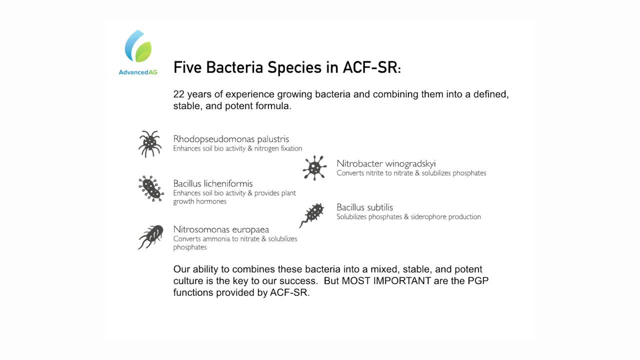 They're plant growth hormones of various types. Then we have all sorts of indirect plant growth promoting functions, sometimes antibiotics, Hydrolytic enzymes- we'll talk about quite a bit, because these are what take complex organic materials and break them down into simple sugars or simple amino acids, et cetera. 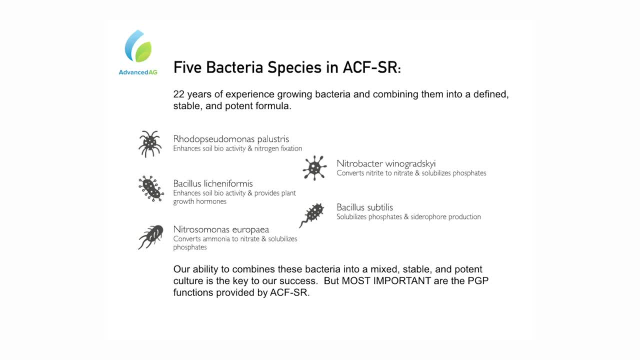 And it turns out that whether you're a bacterium or a fungal organism, you have to have the real simple stuff, Otherwise you can't eat it. So that hydrolytic enzyme is very important, and there's all kinds of documentation of improved disease resistance and so forth. 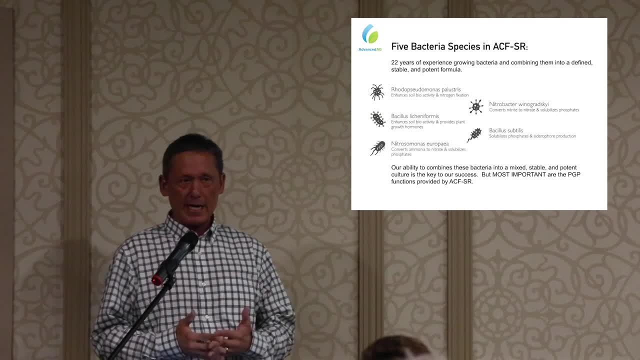 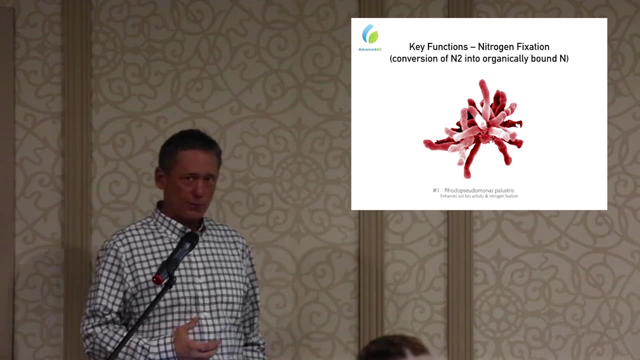 That's starting to make the transition to functions, and that's again really what I want to stress in this presentation. When we listed the direct functions, the first one we listed was nitrogen fixation. This is a micrograph of rhodosudamone. 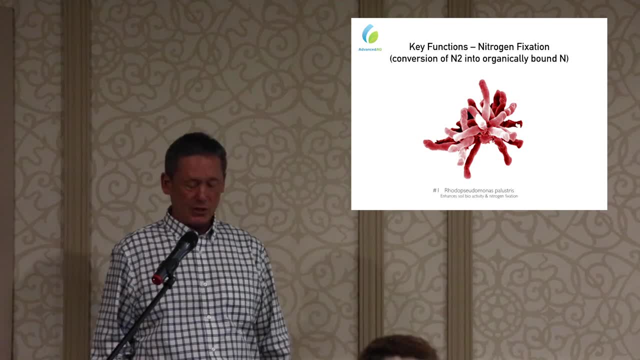 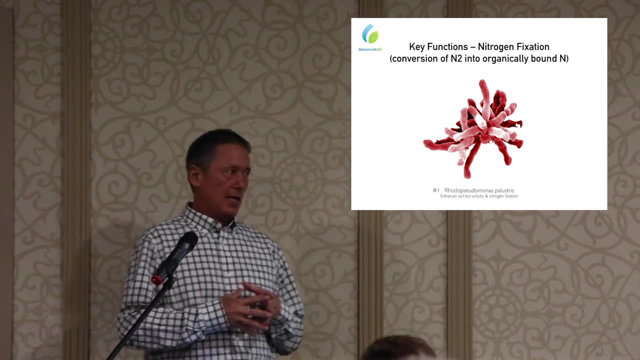 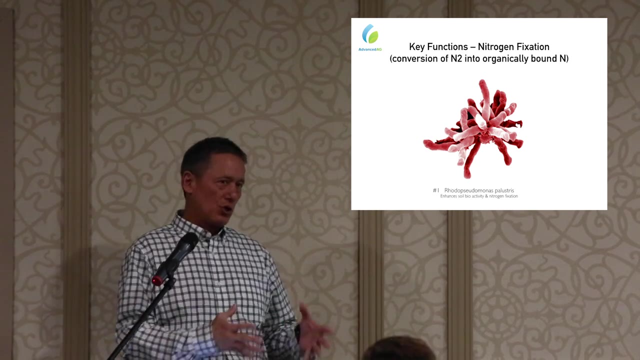 Rhodosudamone, with its red pigmentation, is a very potent nitrogen-fixing organism. You'll see, as we go through this, for any of these species that we have, we can take the identical species and grow it special ways. 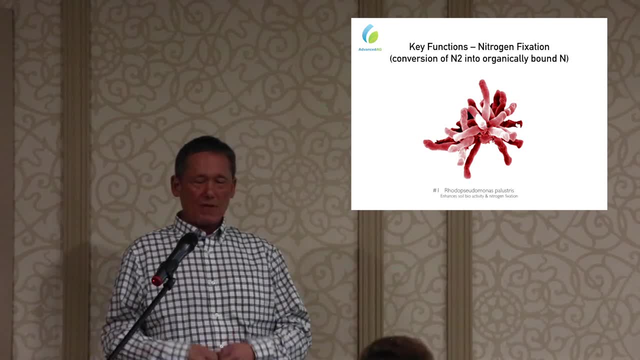 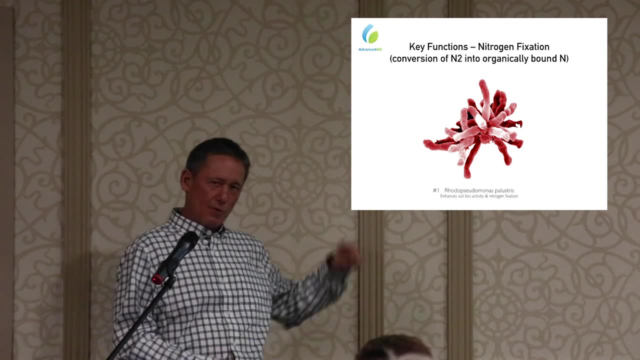 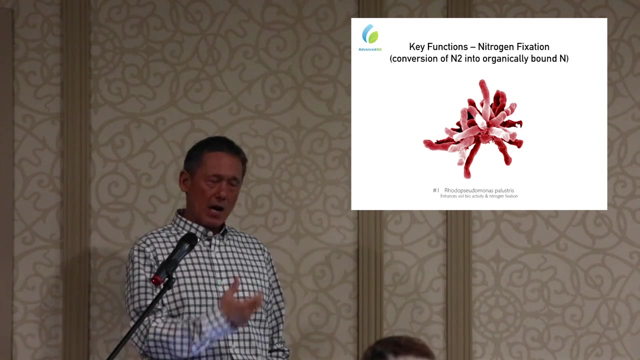 either excluding some nutrients or providing it with what are called inducer compounds, things that we can do to make sure that these important, important functions that we just saw on the chart, that the organisms have that built in so that when they are added to the brew systems. 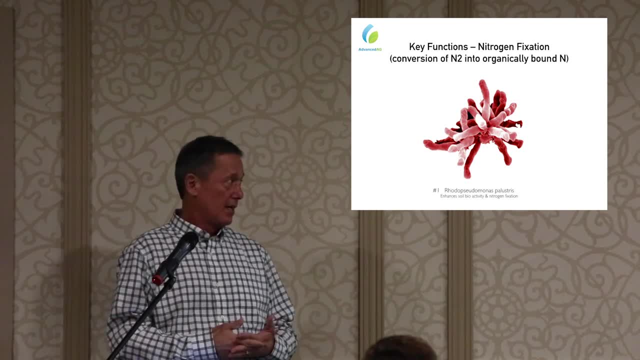 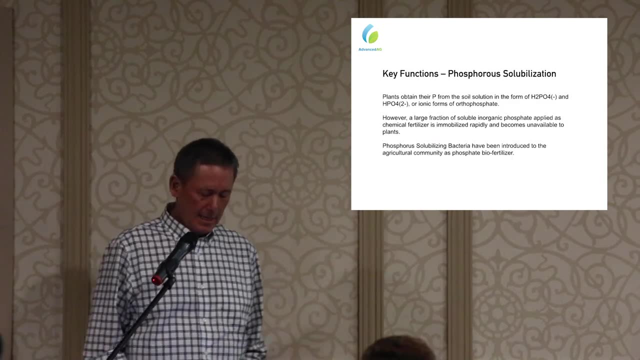 or directly to the field. they provide those functions and it's really, really the key to everything. So the rhodosudamone does a great job of fixing nitrogen, The second main function on here, and we talk about this a lot today. 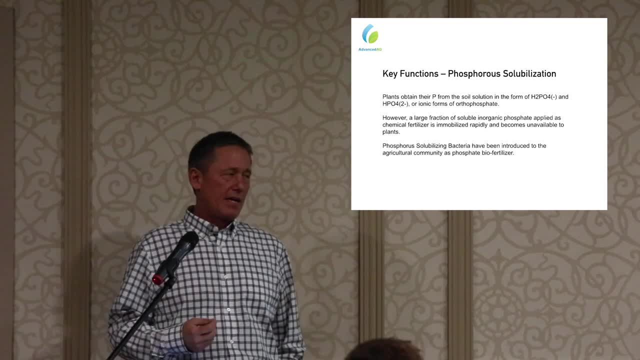 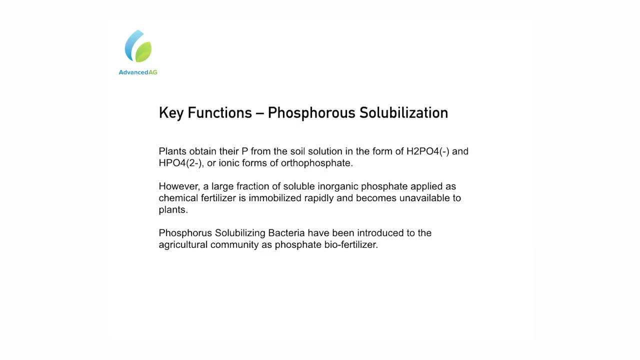 is phosphorosalubilization. Any of the organisms we're talking about- plants, bacteria, fungi- they really need orthophosphate and I think we've all heard these terms a bit. You have bioavailable phosphors and you have nonavailable phosphors. 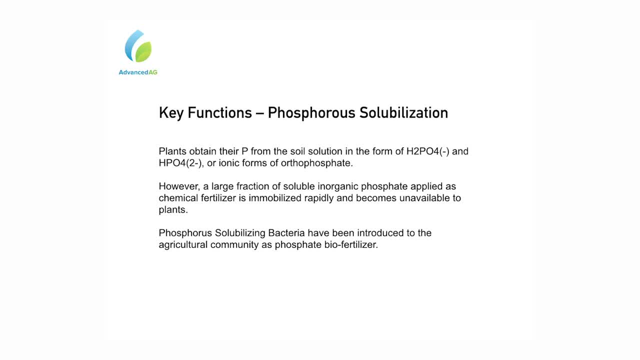 and the orthophosphates, the form it's got to be in a lot of times in soil most of the phosphorus is locked up in a nonavailable form. We have a specific slide on that, but making sure that the culture 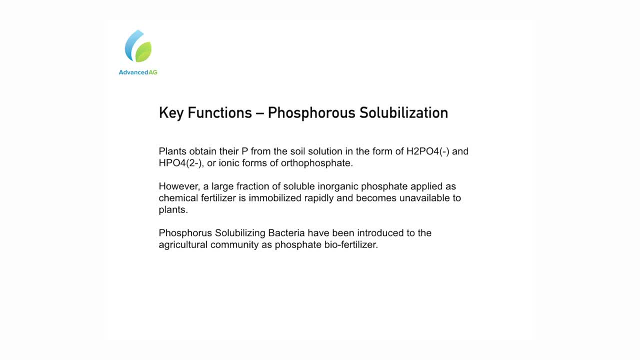 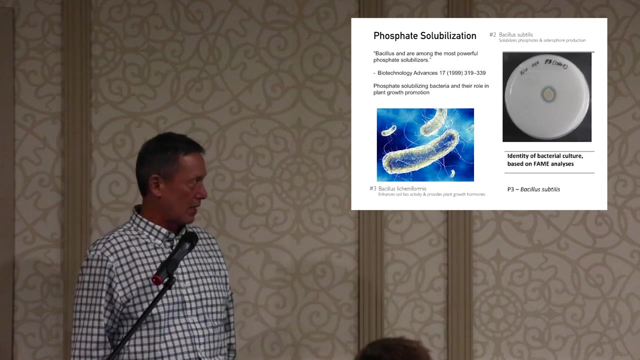 has the function of being able to convert nonuseful phosphors into bioavailable phosphors is one of the most important things that we make sure we keep in the product. Just some examples of how you can do it. This happens to be a bacillus subtilis. 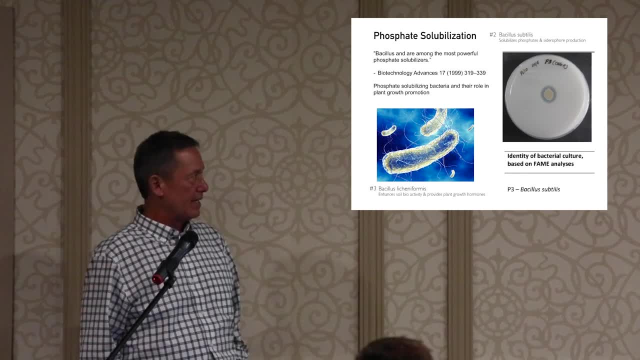 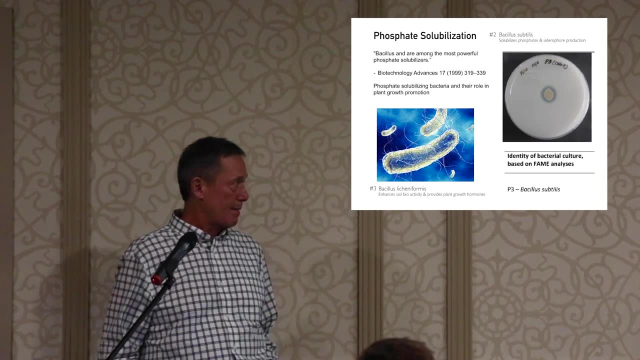 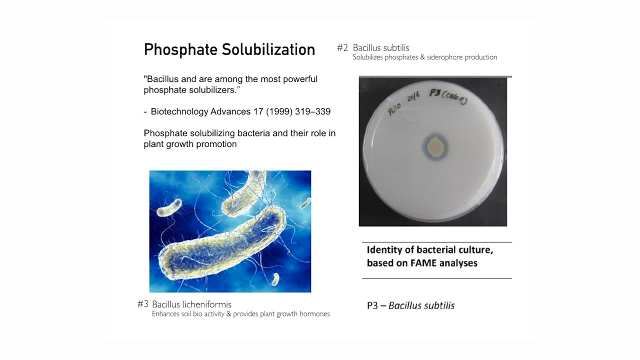 The petri dish on the right side of the chart there that has tricalcium phosphate, TCP, in the plate media And it's not soluble. it's insoluble. it looks like chalk when you have a pure supply of it. 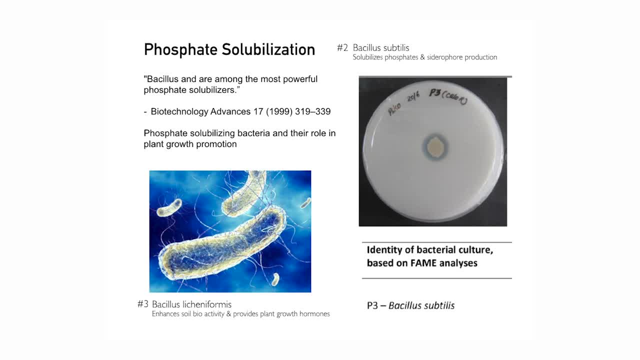 And when you grow the organism on it without other phosphors available, it can dissolve the TCP And when it does that, it has that little halo or clear zone around it. You see the actual colony in the very center and you got a halo around it. 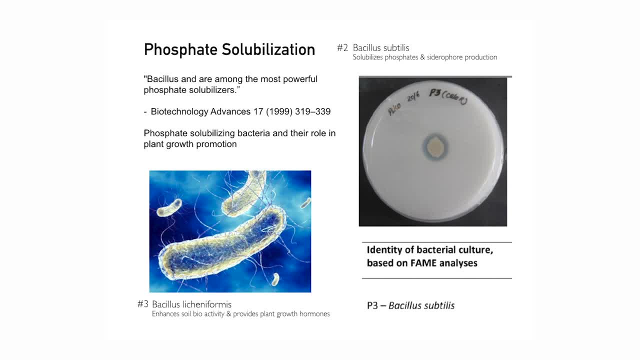 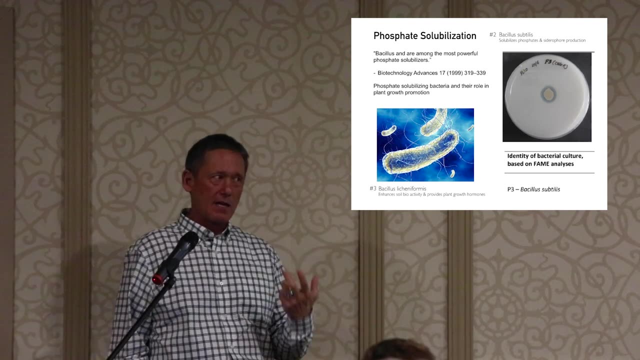 And the size of the halo is directly proportional to how well that colony is breaking down the nonavailable into bioavailable phosphors. So we have about a million tricks like this figured out over the last 30 years, but they're all important. 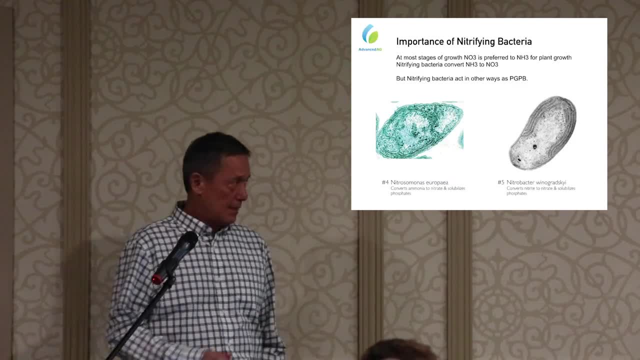 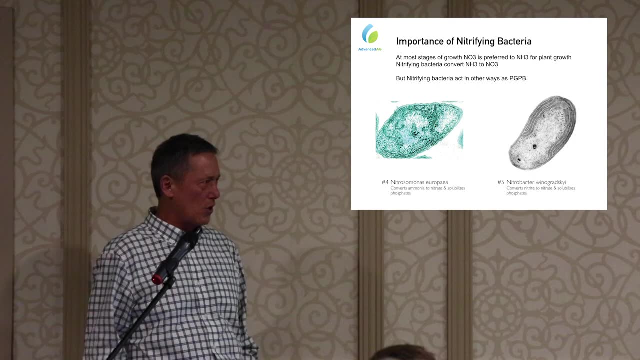 I'm only going to give you a few examples: We talked about the rhodosunomonas and then we talked about the bacillus, the nitrifying bacteria. I think everybody knows it turns ammonia into nitrate and into nitrate. 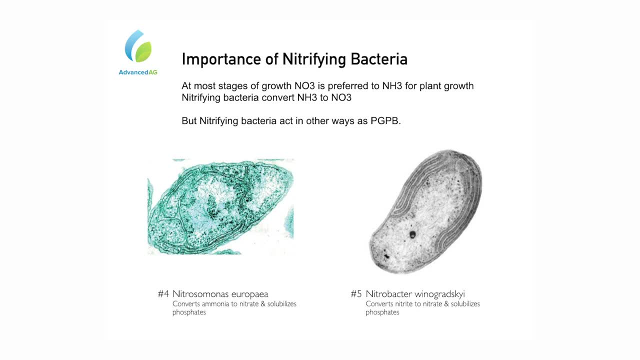 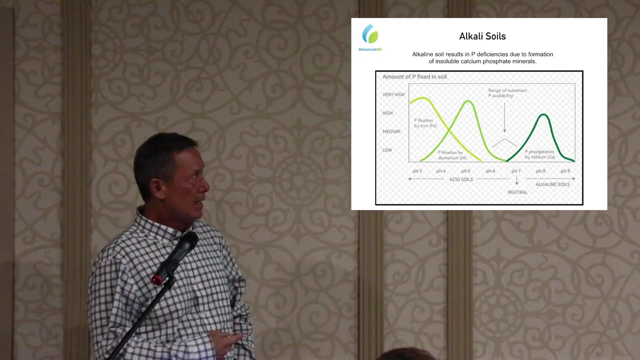 that we found is that there's also some plant growth promoting properties with this, with the nitro fires, and it helps with the phosphorus solubilization as well, and we'll talk about that a little bit more in a minute. this is a really key chart. you've probably seen this in your old 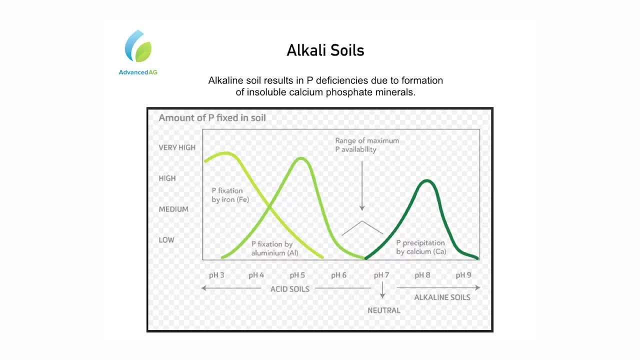 agronomy textbooks. p fixed in the soil. what that means? it's not available. you can't use it. when you have acidic soils, you get aluminum and iron precipitates. phosphorus is bound that way. when you have alkaline soils, you get calcium precipitates and in either case it's not in. 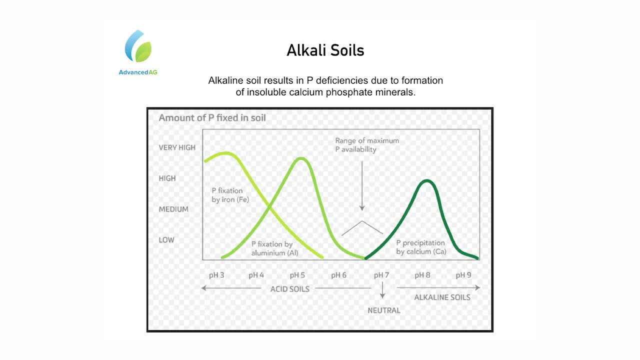 available form so you can add as much phosphorus as you want into a really acidic or a really alkaline field. and even if you're adding orthophosphate, the most expensive form, it'll get bound up pretty quickly and and not really be available. so you know, this is one of the things that we we're really trying to overcome. you see, a little narrow. 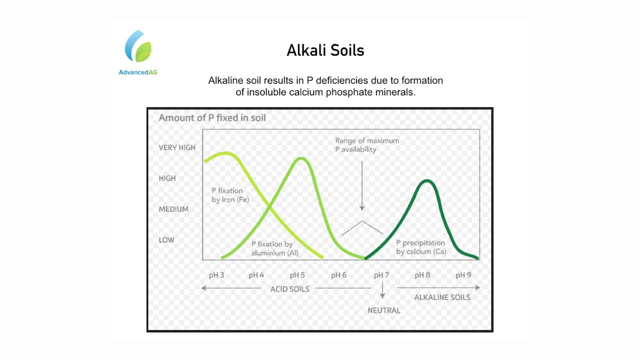 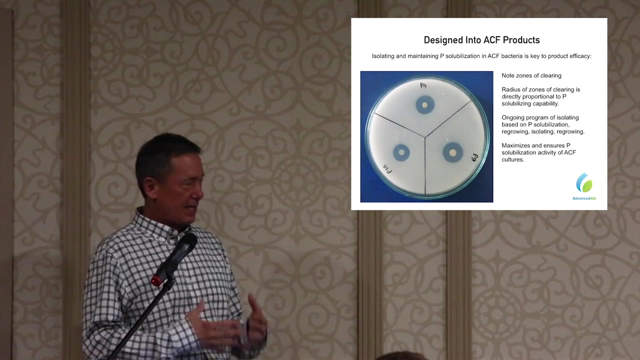 band there where it's soluble, where it won't bind so much, and that's at a pretty narrow ph zone. so it's it's a real limitation that we have in our soils. now in the acf products we can take any of those species and again grow them certain ways, and we do a lot of things such as growing. 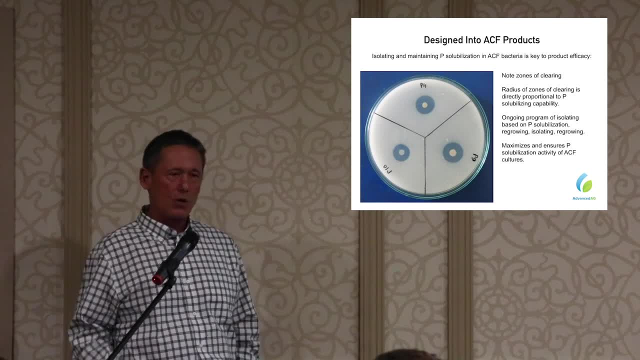 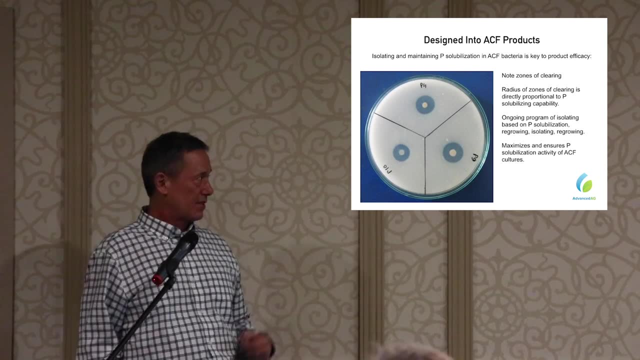 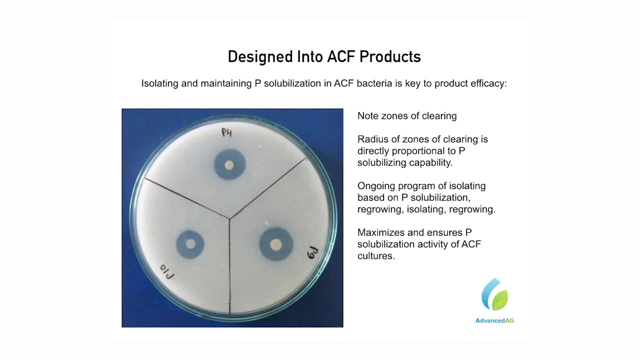 more green plants. this is now you know that's got to have more food. when you give vegetables what's healthy when you gain through the the nitrogen changes, that's when you divided those into again the different transforms and fruit yourself. so a visual way to understand it: that's insoluble tcp. on the outside, the colonies are in the center. 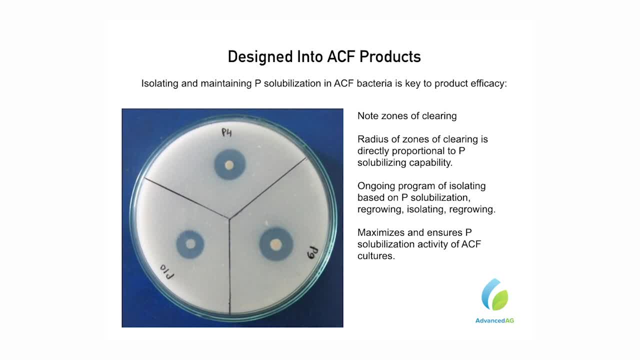 that zone over time at a fixed temperature that's directly proportional to how well that organism is breaking down non-available p into available p. and those are, you know, tricks like that are what give us the ability to ensure that we're putting the functions- not so much the species, but the 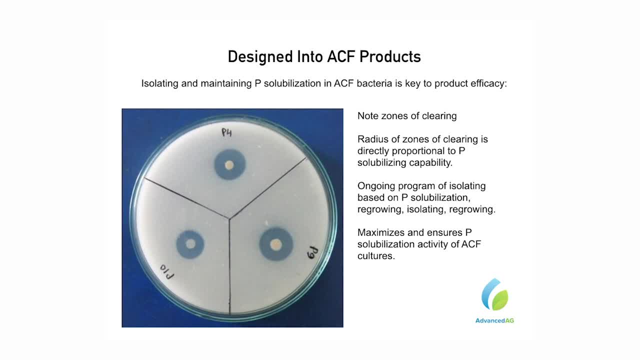 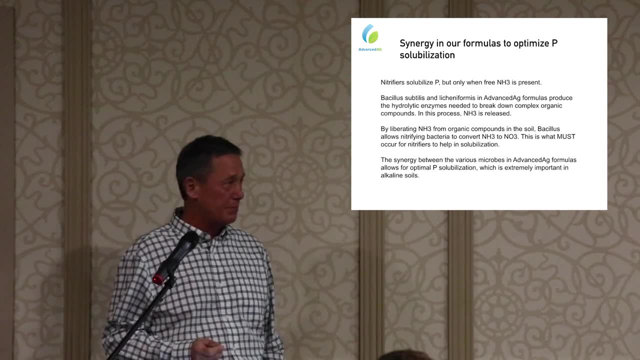 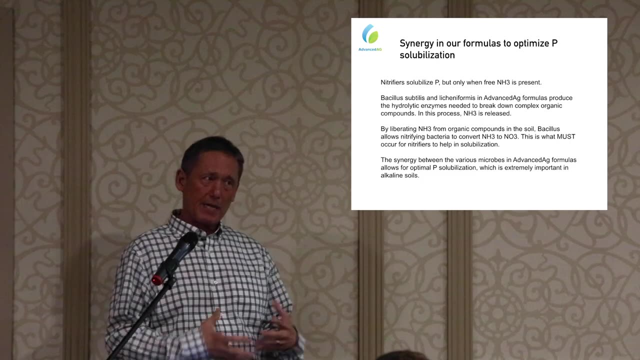 functions into the product just uh, real quickly. one of the synergies that we have is- we talked about these hydrolytic enzymes- if the, if you have proteins or whatnot in the soil, the bacillus can break those things down, liberate ammonia when ammonia is present. not only can you know 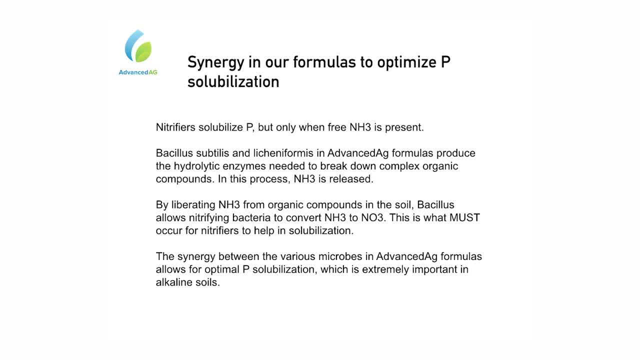 in early, just post germination, that ammonia is taken up by the plants but then a nitrifier can convert it into nitrate and in the process the nitrifiers are enhanced at breaking down and insolubilizing p. so that's sort of a little cycle that we have. the whole thing works really. 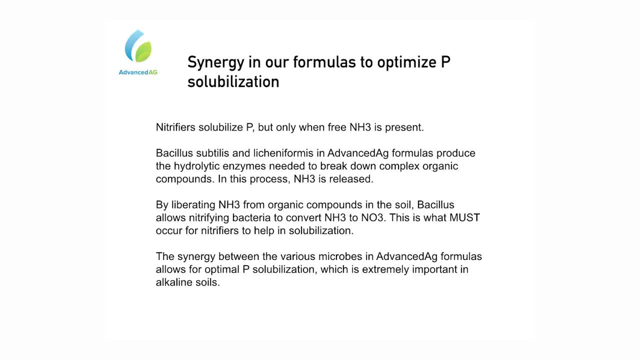 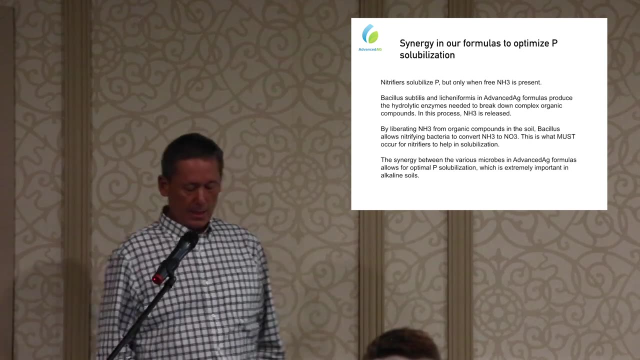 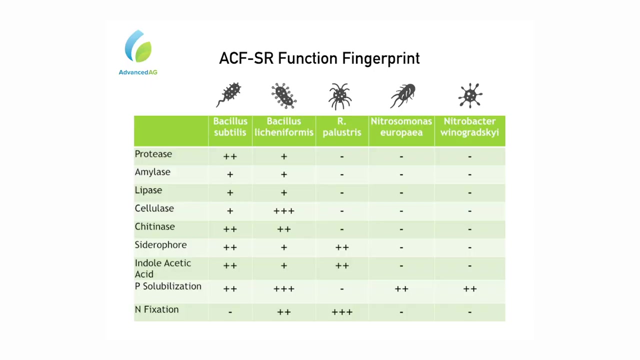 well, but you know there are many species that can do that. but we make sure that we have a defined rate at which we can break down the insoluble phosphorus and make it bioavailable prior to adding that function into the soil. so, having said all that, here's what we we consider our function fingerprint as we look down. 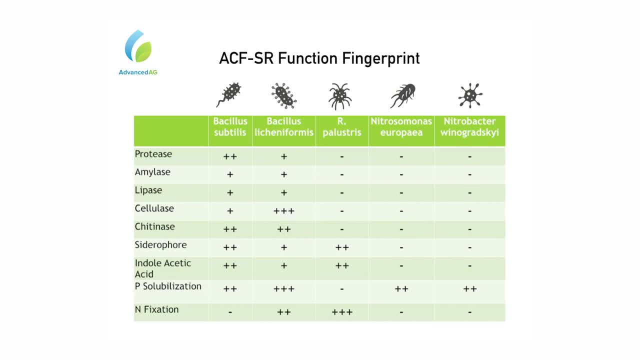 in the very first column we have a bunch of important functions and then, going across, we have the five species that we talked about and you notice some of them do different things. for example, the first one, the subtlest, is really good at making protein documentaries. they're a prominently joined group with other species. that's what we're interested in doing in plants, but also色 Alec and save borax, come on. what else in other featuresAKE, HERETICALS, i don't know, but i would hope theyraz and other plant protection groups to do so, because i know that. 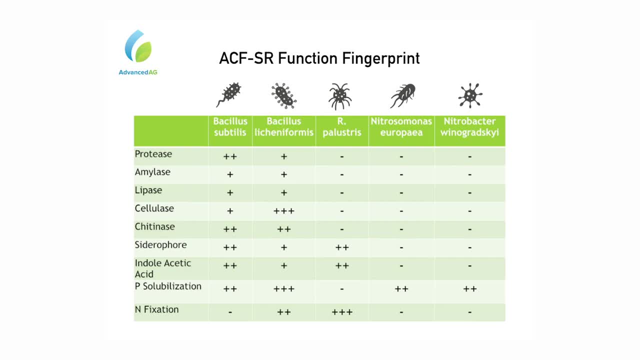 digesting enzymes and it's pretty good as we go down with more plus signs. And you know all of that can be done, but only using, you know, all these tools that I briefly illustrated, with those zones of clearing on the phosphors. 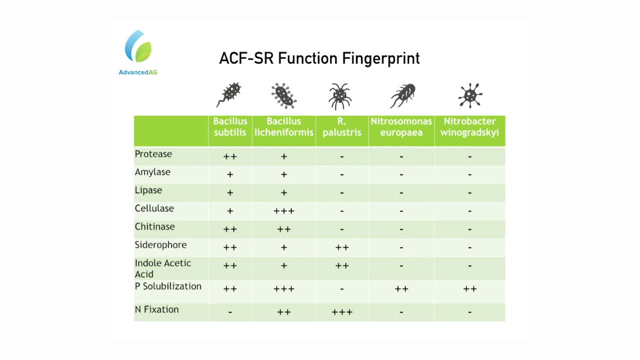 So this functional fingerprint, the transition we need to make when we're thinking about what we're adding in terms of a probiotic to crops, You know, does it matter if we are adding the species, if they grow or not grow, That's not so important. 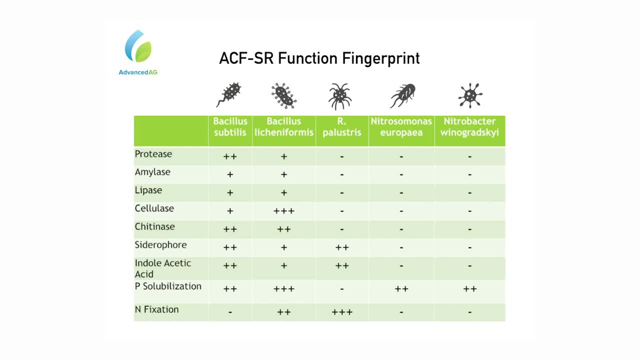 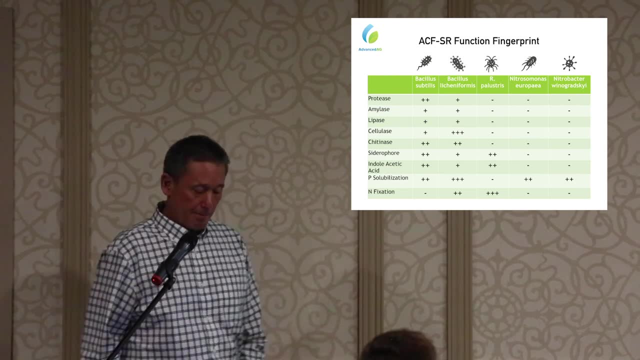 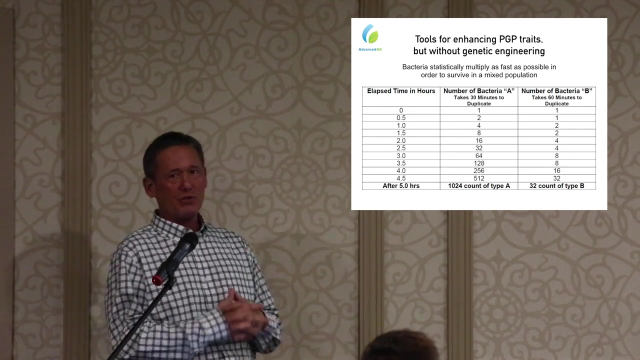 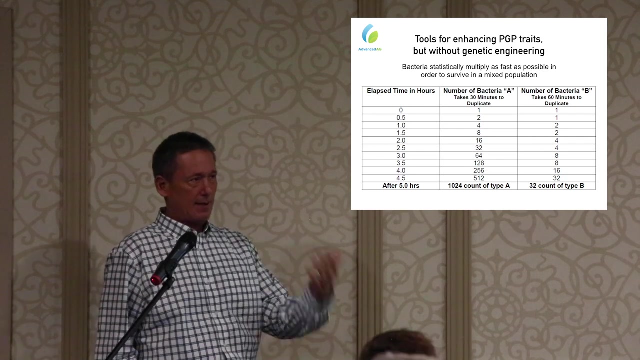 What's important is that we're adding these specific functions into the soil, and we will talk about why that's important based on this type of chart. Well, fungi reproduce differently. Bacteria: they split by fission: One turns into two to four, to eight, to 16, et cetera. 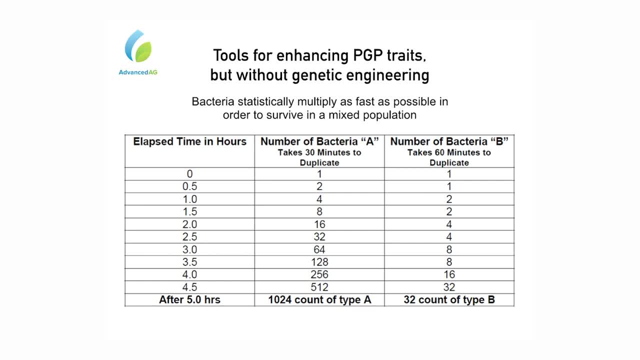 And this is just an example: The center column in the chart, that's bacteria that reproduce every 30 minutes, And then on the right-hand side, those are bacteria that reproduce every hour. After just five hours, you have 1,024 of the fast growers and you got 32.. 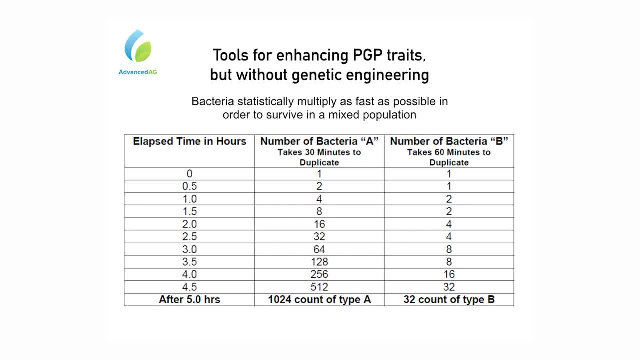 Now you can understand, in any mixed food environment, whether it's on the field or in a beer fermenter, anything by species that's growing faster is going to quickly dominate Here. in this situation, you got, you know, 0.3% of the slow guys and you can imagine. it. If you take it out a few more hours, it's really easy for the slow reproducing organisms to get lost, And it's just a matter of who's going to grow the fastest, And it really is literally the survival of the fastest. 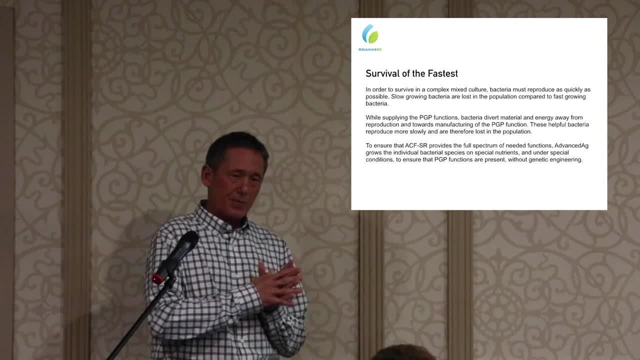 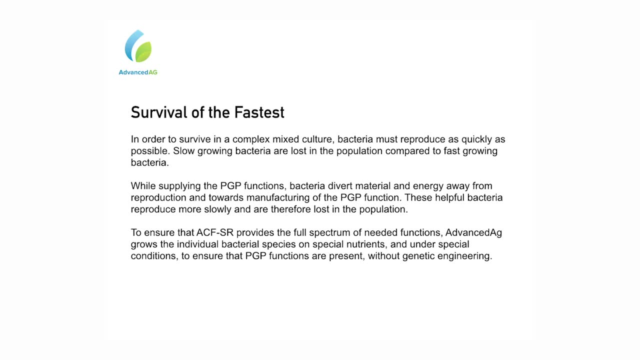 And what we want to talk about is all these different functions, all the different efforts that we put into making sure these bacteria can make protein. They're degrading enzymes and chitinases and plant growth hormones. While they are doing those things, they're using the material and energy that they have. 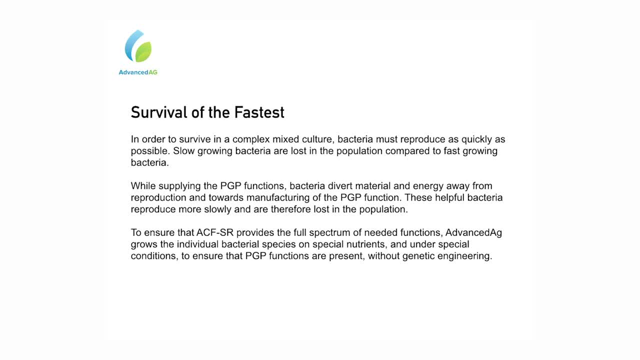 to produce those products, those functions and their reproductive rate slows down. It's literally just by definition. if you're making things that aren't directly related to your reproduction, your reproduction rate It's down because you only got so much material and energy left. 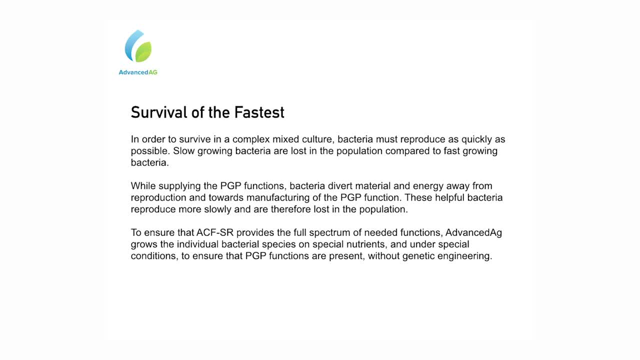 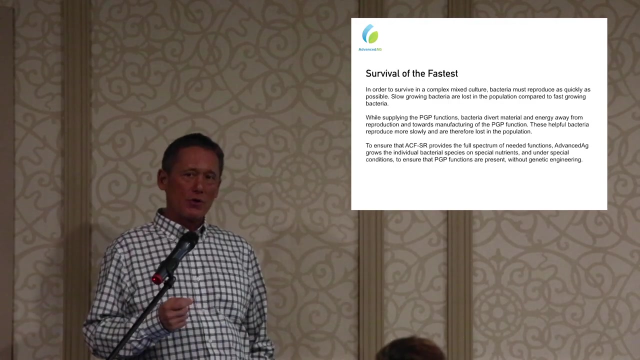 So, without a doubt, when you have a culture that is producing all these additives and the functions and the enzymes and everything else that we showed in our fingerprint chart, their reproduction rate is low and that's unavoidable. And the organisms that are just growing and reproducing without doing that stuff. 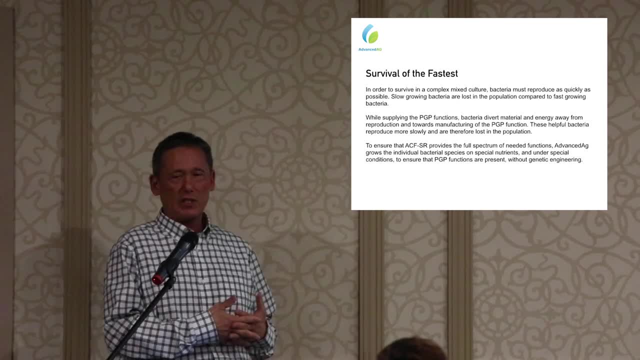 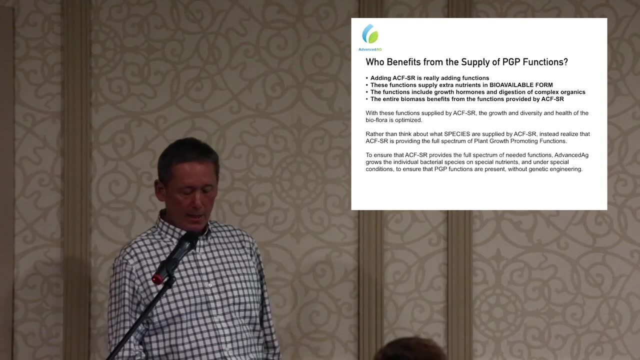 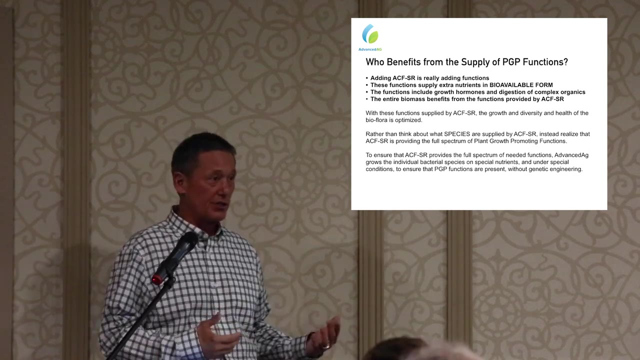 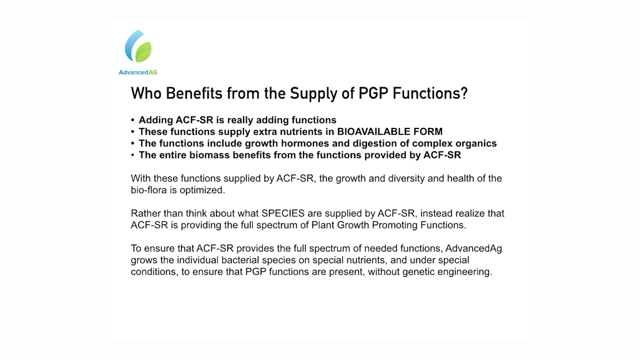 their growth rate is fast. So we just saw 1,024 versus 32 in five hours. So we can all do that math. Now, who or what benefits from the supply of all these plant growth-promoting functions? And now we're really making the transition from talking about bacteria or fungi to these functions. 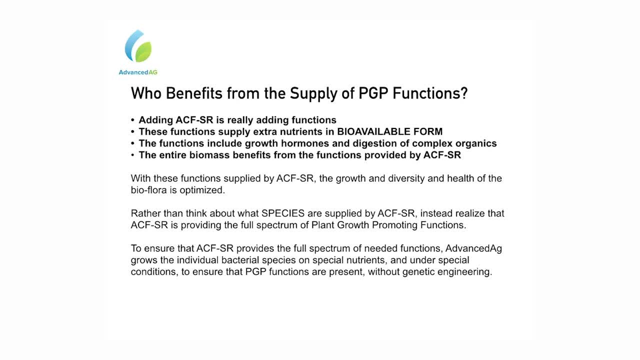 When you add these functions into the crop, you're not really adding the species that are generated in that brew tank. We know what they are, We can count them, But what we're really adding is the functions, And those functions. they provide extra nutrients, whether it's simpler organic compounds or fixed nitrogen. 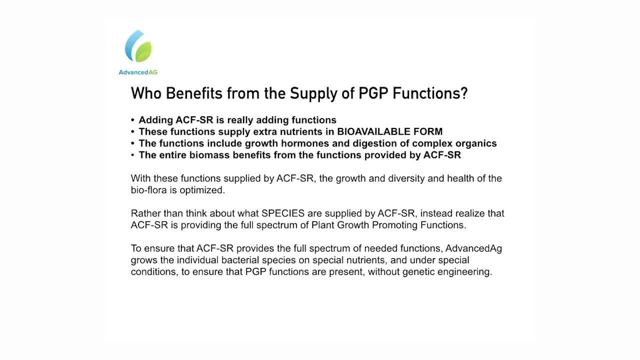 or more available P. Who or what is going to take advantage of that? Well, it's going to be anything that's in the location where those nutrients are supplied. So all of those functions, including the P-solubilization, the growth hormones. 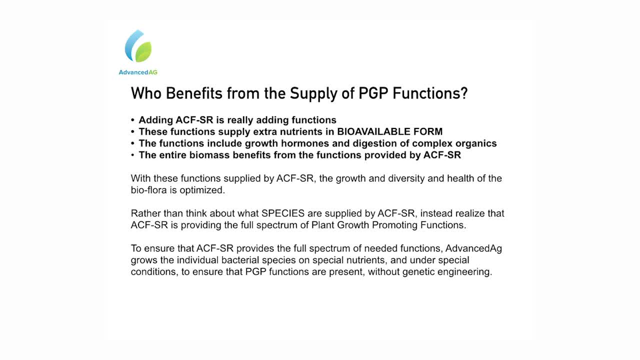 the entire biomass benefits from that And it's certainly not. you know just the organisms that we're putting in there And you know we've done a lot of studies of tracking the populations of different things over time. you know post-inoculation. 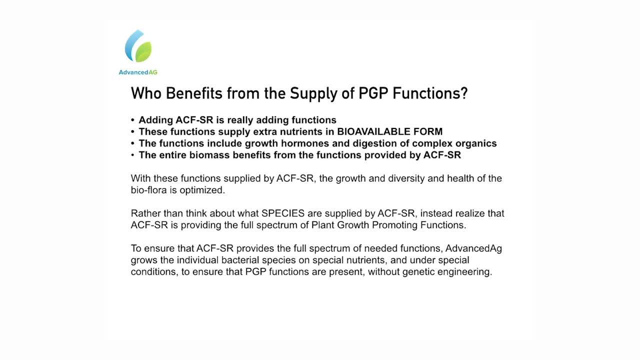 And invariably, what you find is that we see the numbers of what we put in, because we put it there, you can measure it, But the growth of the other organisms goes up dramatically. Why? Because those promoting functions boost the nutrients, the hormones, the increased available P. 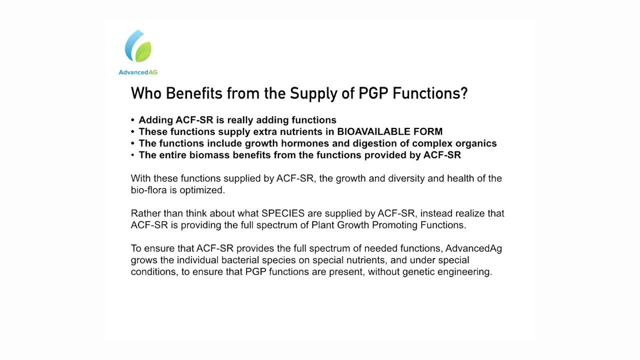 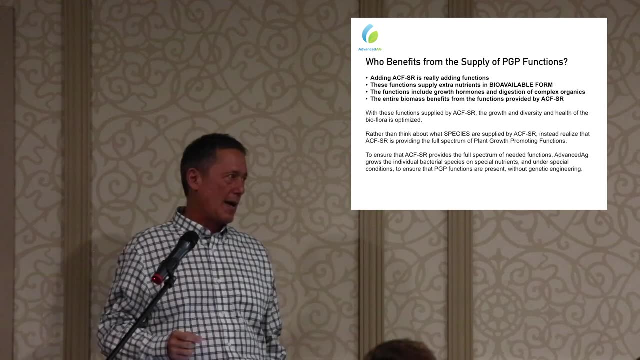 et cetera, for everything that's in the biomass. So this is never a case of adding our bacteria and they take over the crop Or they take over the ground. It just doesn't work that way. We're literally putting in functions rather than numbers of bacteria. 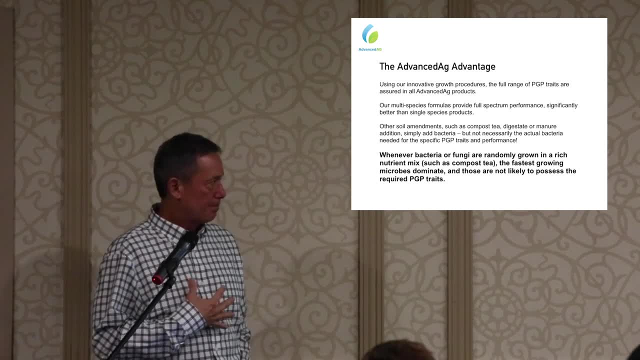 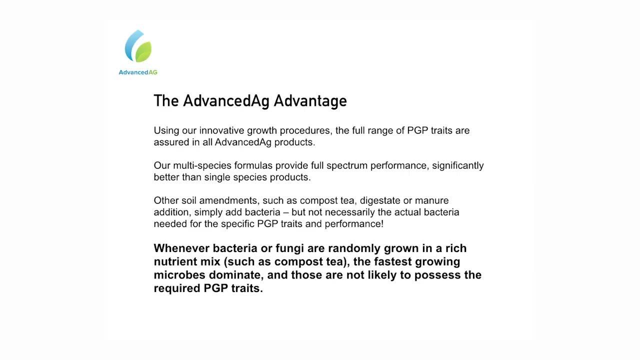 So our real advantage is that anytime organisms are grown as fast as you can in a molasses broth or anything like that, or compost tea, and people are just trying to boost bacterial numbers or fungal numbers, all that you get are organisms that can grow fast. 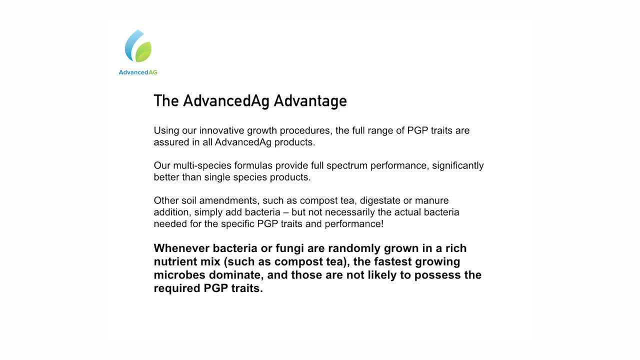 They are not necessarily producing any of the useful functions. They're not really delivering anything. You can have 10 to the 9th or 10 to the 13th, it doesn't matter if they're not doing the things that break down the phosphorous, that fix the nitrogen, that break down the complex organics. 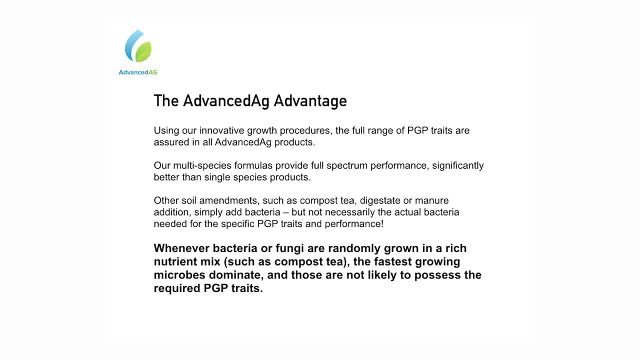 And the fast-growing organisms don't do a good job of that. So you know, we recognize that we've spent literally 30 years- you know years- figuring out how to confer enhanced functions on the culture and then how to take it into the brew tank, which we're anxious to unveil and make it economical. 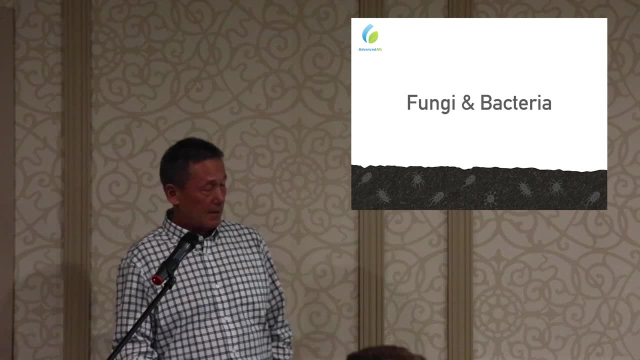 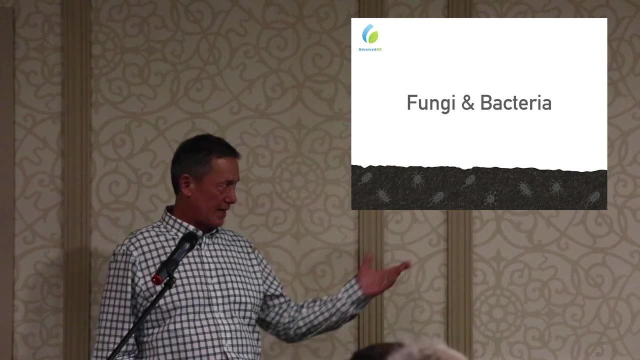 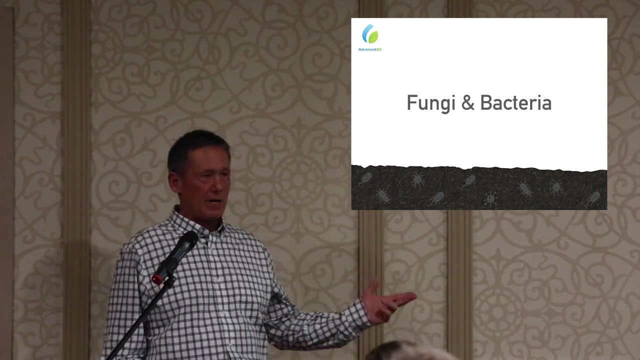 and predictable for everybody. Having said all that, I do want to say a little bit about fungi and bacteria. You hear a lot of people- and I think Joshua alluded to it earlier- that you have- well, I have- trichoderma. you don't have that. 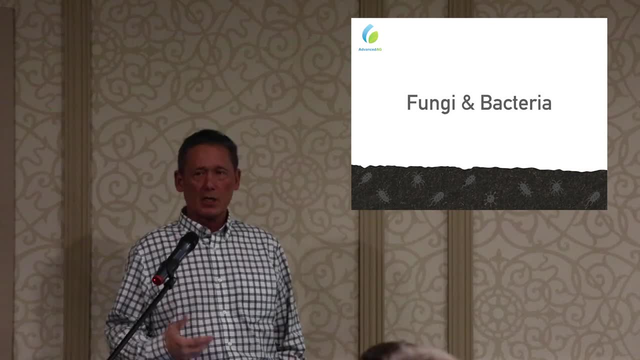 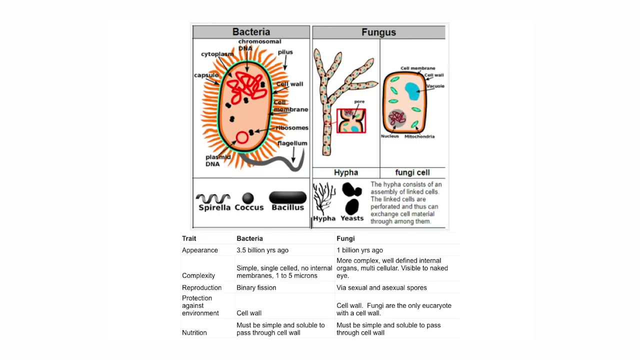 Or we have, you know, whatever count. You know what does all that mean? So I'm just going to compare and contrast fungi and bacteria for a bit here. Bacteria on the left- this is not to scale. Bacteria are really small. 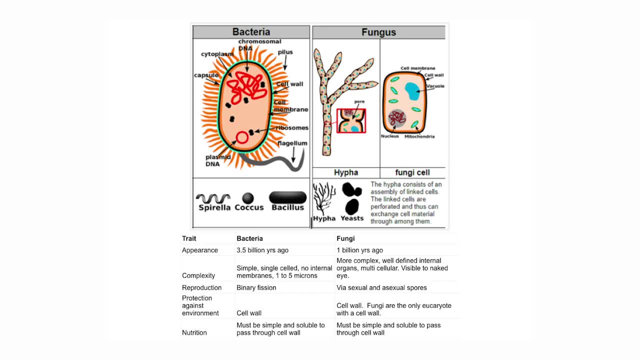 Fungus are larger and some occupy entire forests. You have: bacteria were around about three and a half billion years ago, as opposed to about a billion years ago For fungi. we already talked about the reproduction. Bacteria split in two, into four. 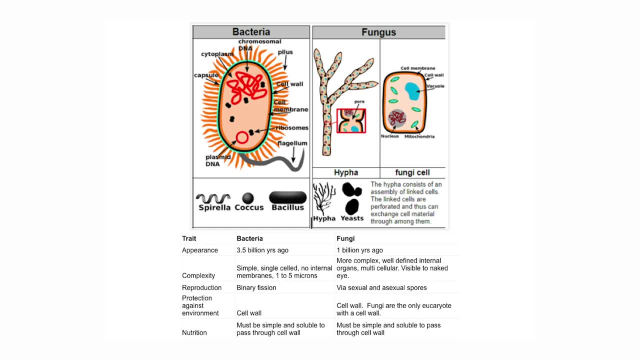 Fungi have both sexual and asexual growth and a very different situation there. One of the things that's very important is this: protection against the environment. A cell wall is something that surrounds all bacterial. It's a semi-permeable membrane. It prevents complex stuff from getting inside. 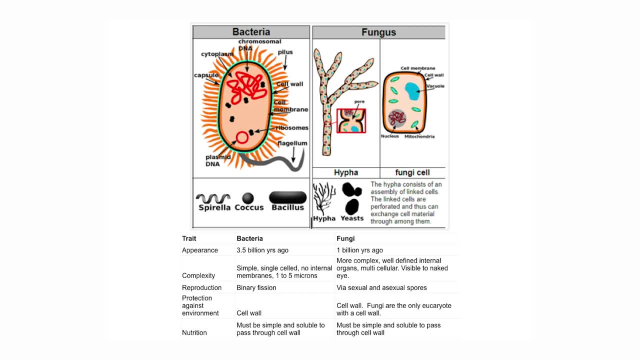 So the bacteria have to have simple stuff to eat And fungi as far as complex organisms. they're the only complex organism that has a cell wall, And that's also important because, just like bacteria, fungi have to have simple soluble material as a nutrient source. 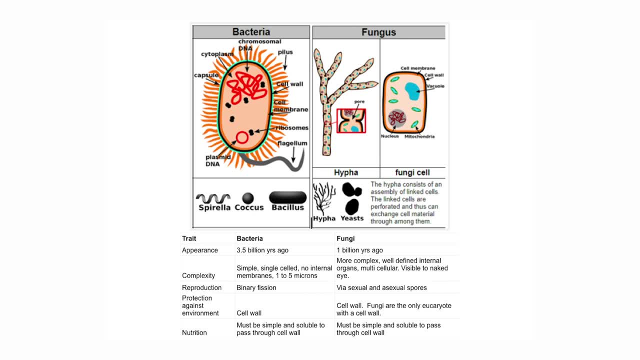 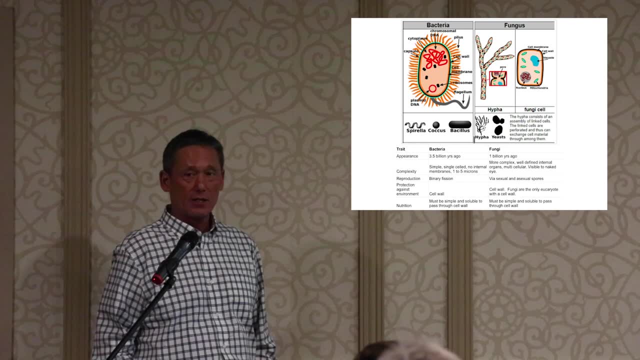 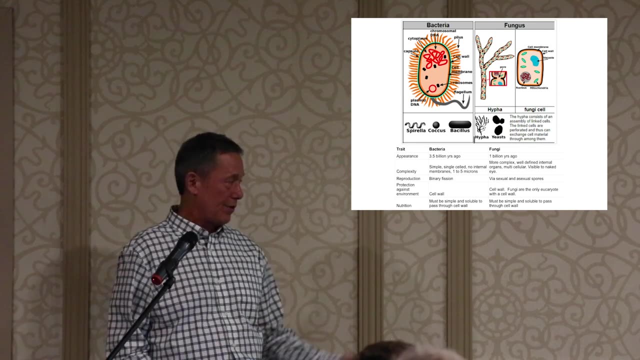 Just to give you an example of what we're talking about: the major protein in milk, casein, is too large to pass through the cell wall of either the bacteria or the fungi, And that casein has to be broken down into its constituent amino acids before these guys can eat it. 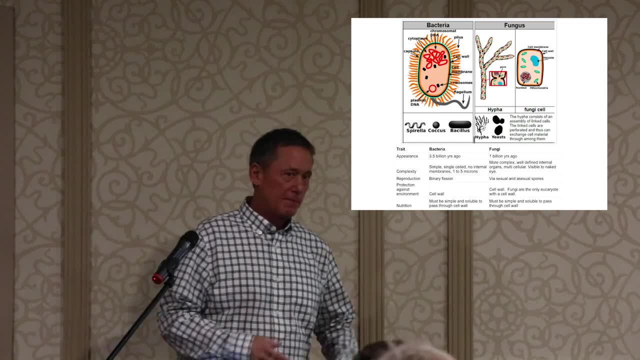 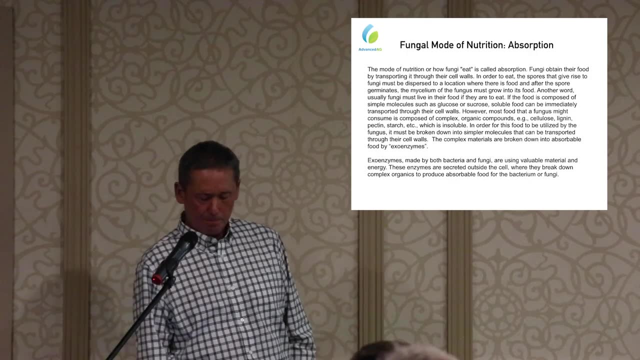 So even something that you might think is soluble, like milk, is not for the purpose of these organisms. They have to have the simple soluble materials. Another factor is: 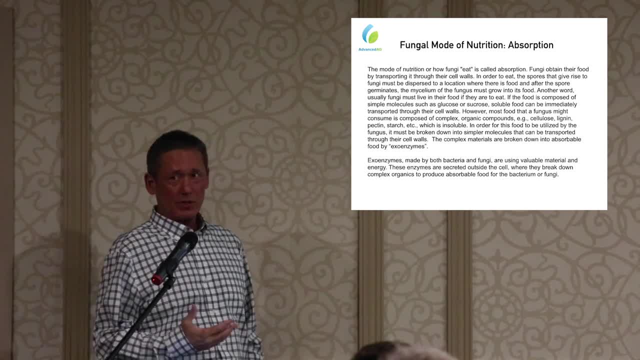 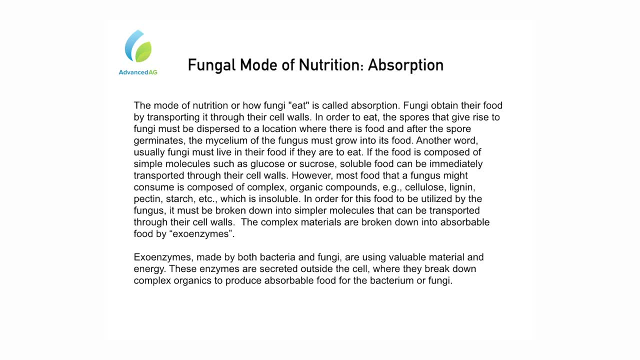 I've seen some good results from adding fungal products, but, having said that, they're all supplied, generally speaking, in spore form. 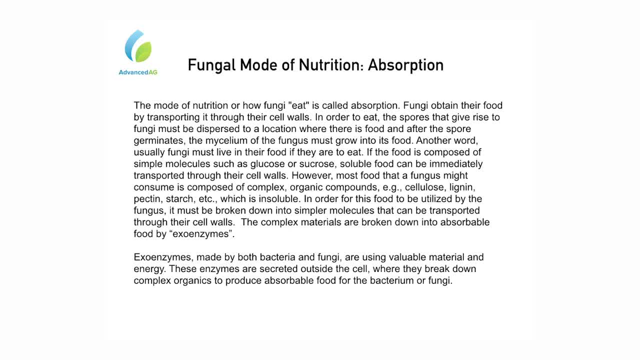 Spores have to germinate. What allows spores to germinate? Well, it's a complex variety of things, But for one you have to have nutrition, which means you have to have the soluble organic compounds, And then there are all kinds of other conditions for specific fungi. 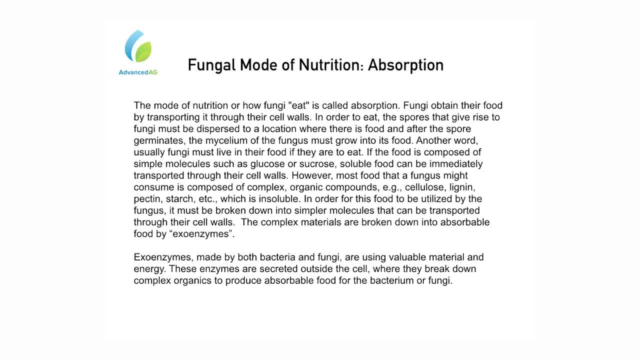 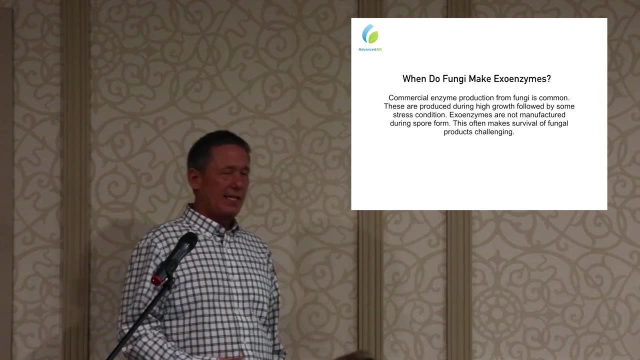 But it's not super easy. The mode of nutrition, just like bacteria's absorption. you have to have the simple, soluble stuff, or the fungi can't touch it. It has to get through the cell wall, It has to be soluble, So both bacteria and fungi can make these enzymes inside themselves that they excrete. 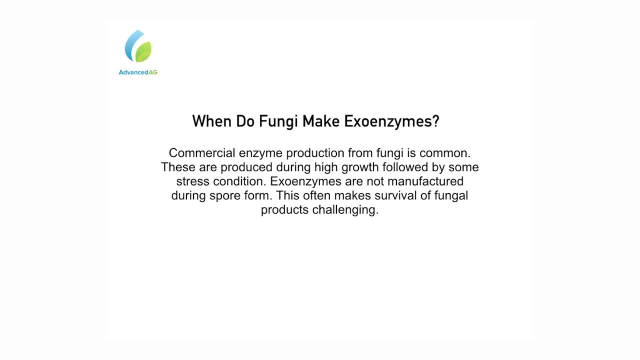 into the media And that breaks down to complex stuff And that gives them some soluble food. That's the only way they can grow And, as we talked about before making these enzymes, it doesn't help that organism grow. It slows down their growth. 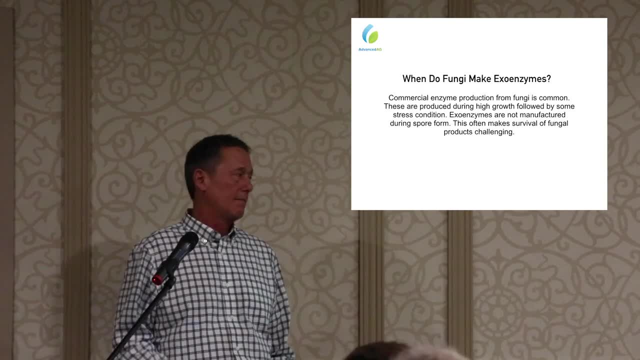 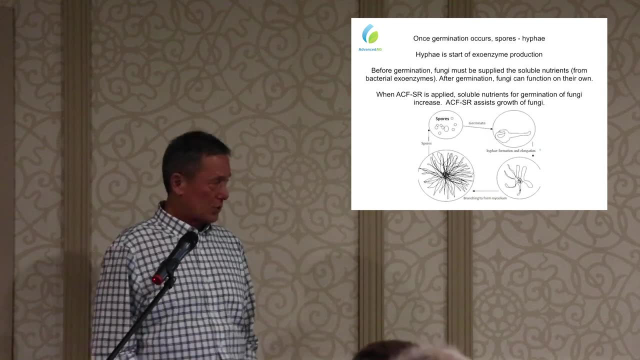 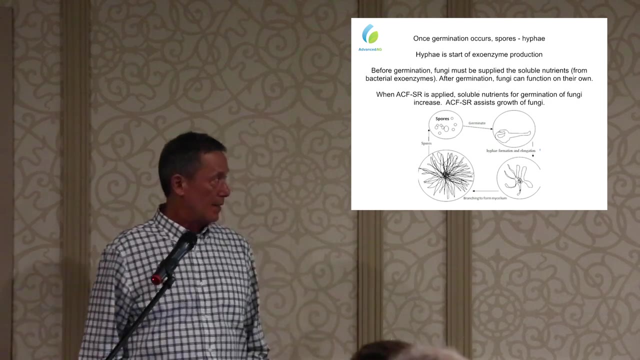 So you know it's not occurring in the soil at the rate that would be optimal, whether you're germinating fungal spores or whatever reason. So fungi can make the exoenzymes. When do they do this? They really do it as they go past germination. 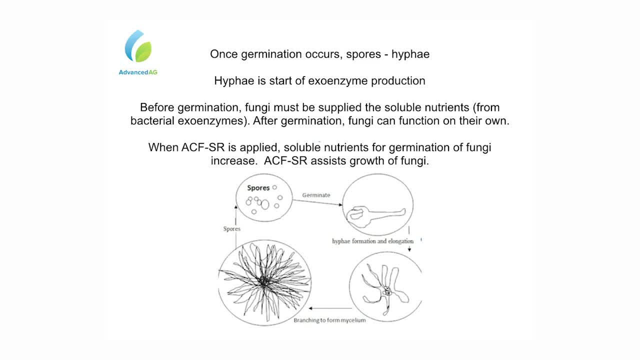 And they form hyphae, which, once you get to that point you know. then they can make the enzymes. But if you're adding just fungal spores, there's no guarantee that they're going to germinate. And if they don't germinate and start to grow, they're never going to make these enzymes. 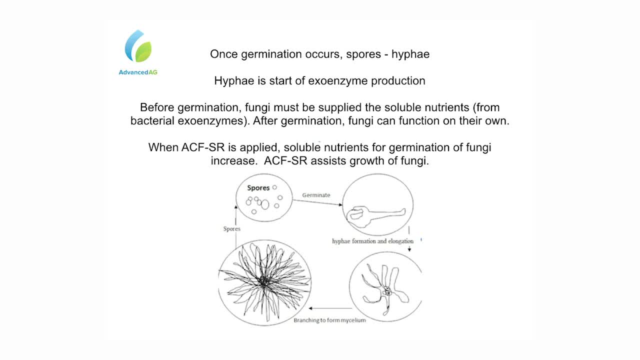 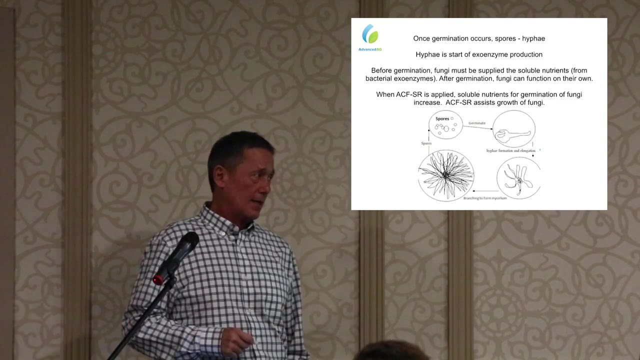 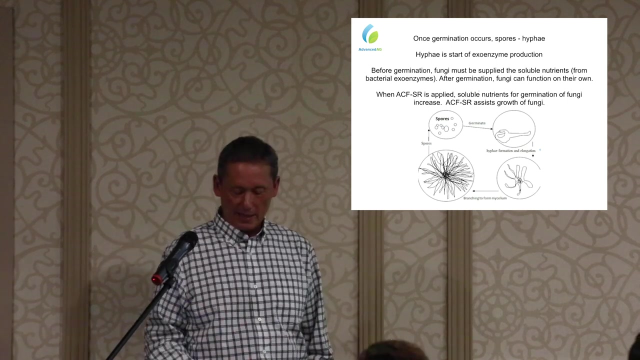 You sort of run into a dead wall. So, and it's never the case that only bacteria or only fungi or only one or two of those functions should be added. It's always a big picture and always a combination of different things. But I'm just pointing out that you can't just take fungus spores and throw it on a field and necessarily expect anything good to happen. 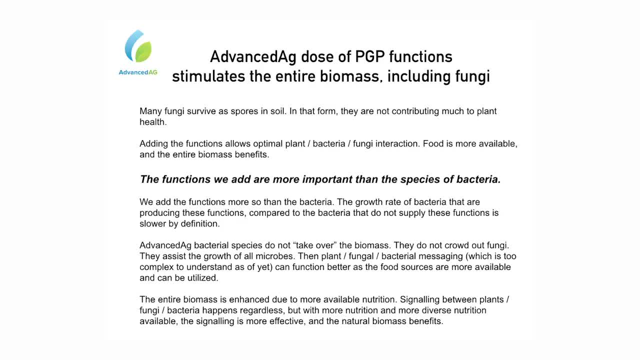 All these words here. I'm not going to read those, but the middle statement in bold: the functions we add are much more important than the species or the numbers. You see all sorts of things about how many. You see a few where you know this. none of that. as far as we're concerned and as far as we've demonstrated, that doesn't mean a thing. 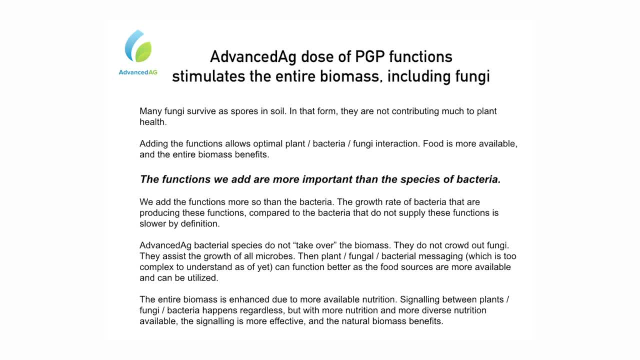 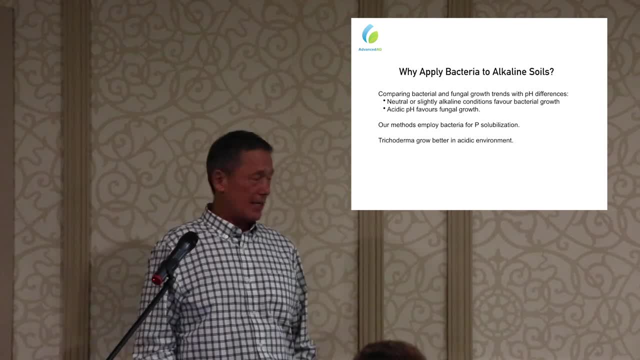 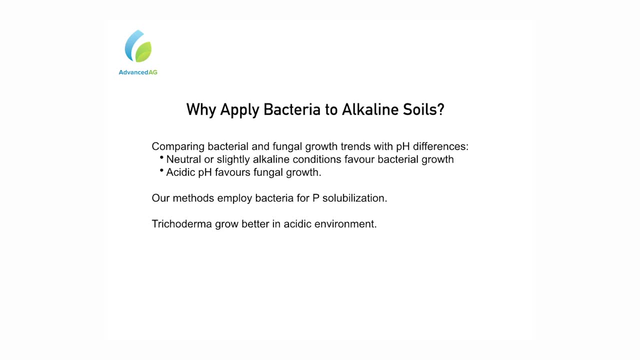 It's: how much activity of the right functions are you adding and at what cost? Here in Western Canada is almost all the soils alkaline to one extent or another, And when you have that type of thing, it has an impact not only on the fungi. 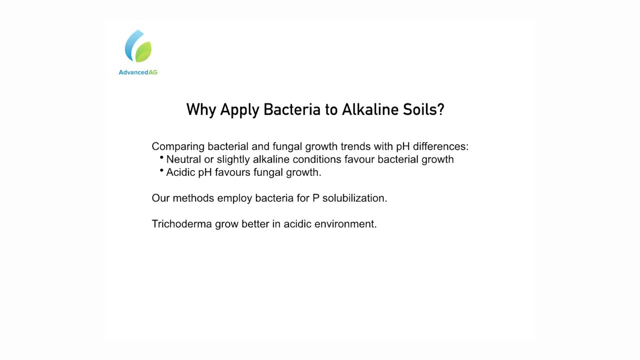 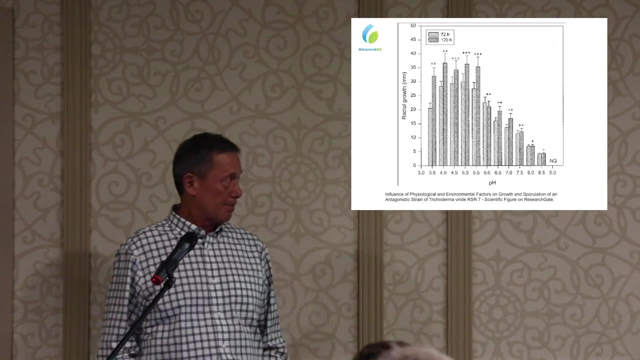 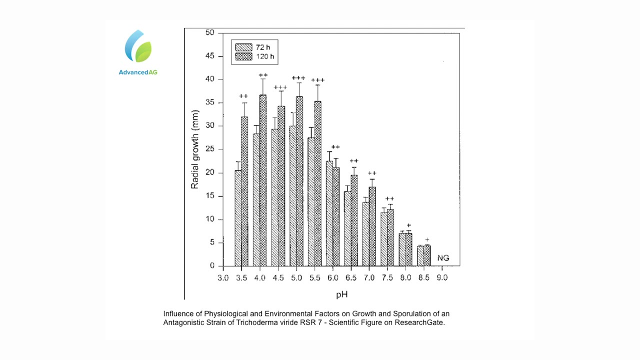 in the phosphorus availability, but on fungal growth as well, And this is just to put everything into context. We have this picture. this is a Trichoderma species at PH, and this was done in a series of plots across New York state. 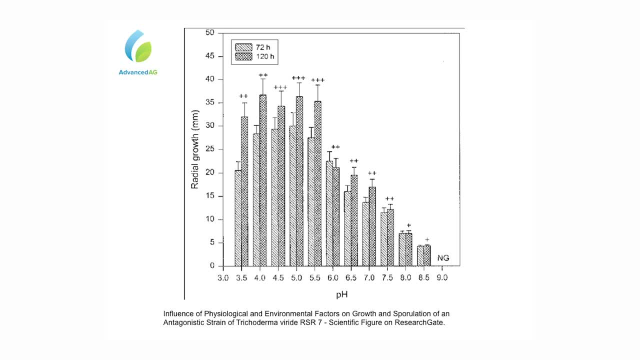 As you can see, when you are at the far left you are at PH 3 and you get up to PH 9, at the far right you have Edition нормально Ph 9 with some sort of frame ring and orazic extension. 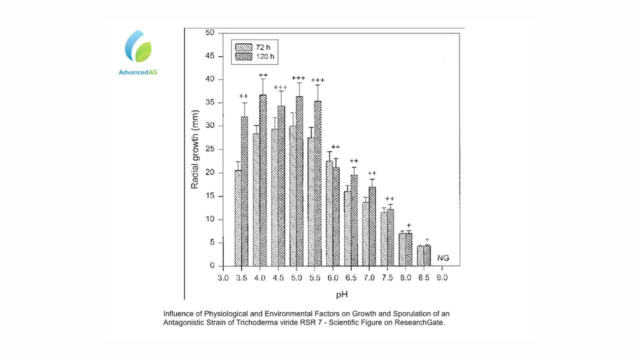 are right. Almost all the fungi, certainly the trichoderma. they have really good growth at a high pH. When you have, you know, forest type soils and you have an acidic pH, or you have a high fungal population. when you have alkaline soils, the fungal population never really gets. 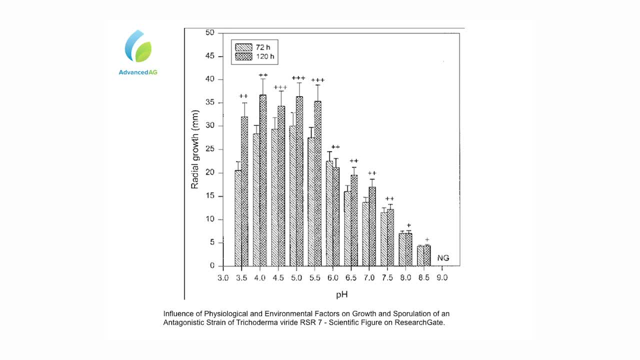 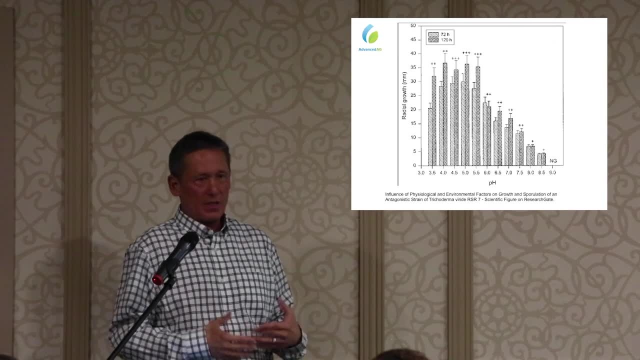 up there And so these sorts of things. it all comes into play when you're talking about: do you want to add bacteria or fungi? And remember what we say is none of that matters. You really got to add the functions and let the natural biomass take advantage of that. 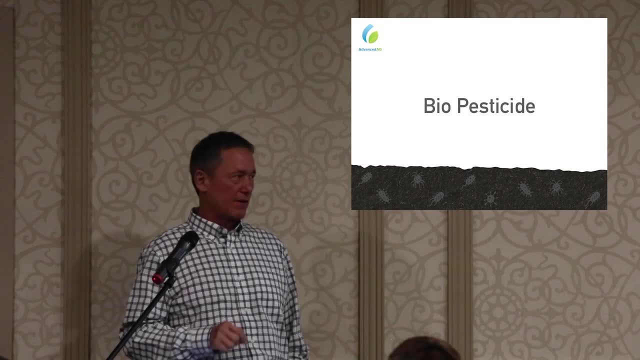 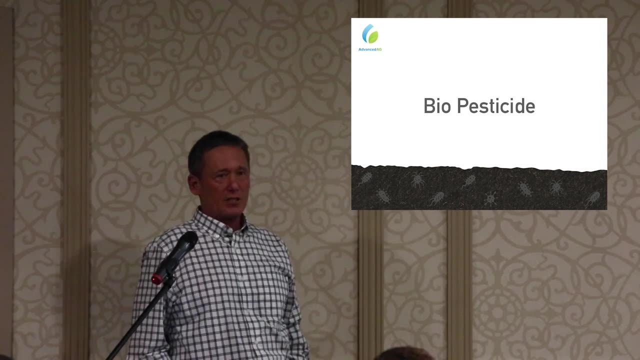 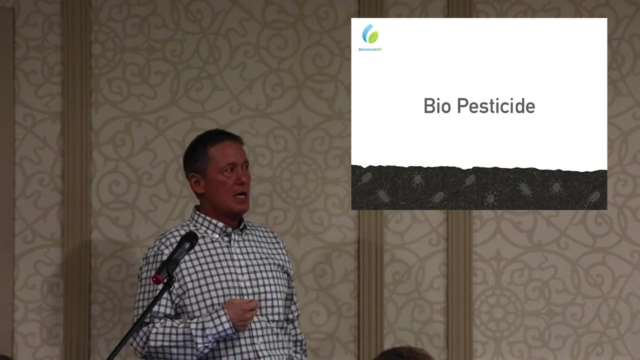 We're going to talk a little bit about something that's coming down the pike very, very soon. For the last several years we've been working very hard on biopesticides that, for one, have some of the plant growth promotion properties, but for two, are really strong. 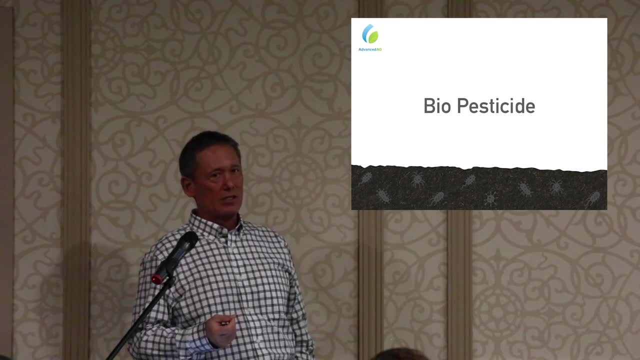 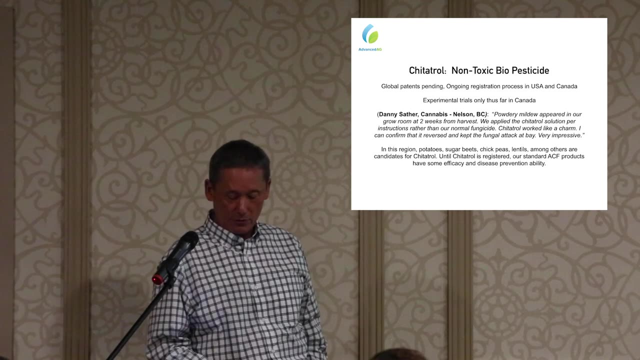 producers of biopesticides, And so we're going to talk a little bit about that, An enzyme that breaks down the fungal cell wall, which is largely made of chitin, and it's called chitinase, the enzyme that's being produced. 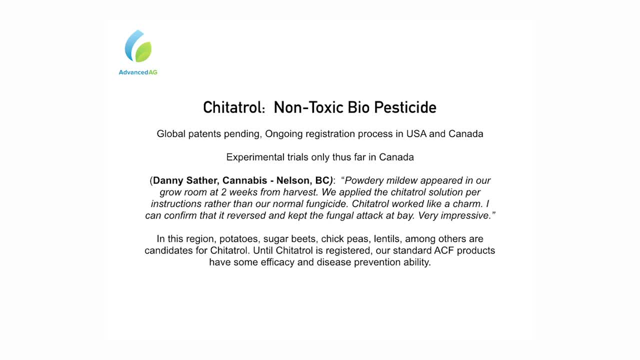 Trade name chitotrol, a non-toxic biopesticide. There have been some spotty trials- nothing that was significant here in Canada, but people have seen some real good results with that. There's been no sale yet because it's not legal. 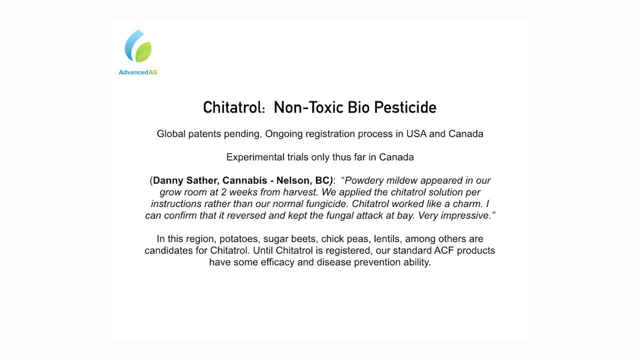 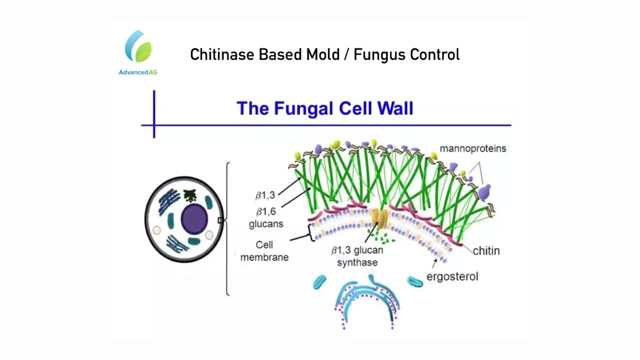 But there are countries where you know we've been able to get it out there pretty well. What we have here is just a diagram. It's just for emphasis so we don't have to worry about all the chemistry going on. but the cell wall is largely made of chitin in fungal organisms. 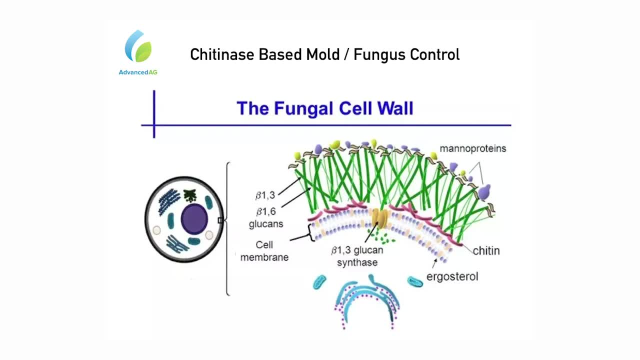 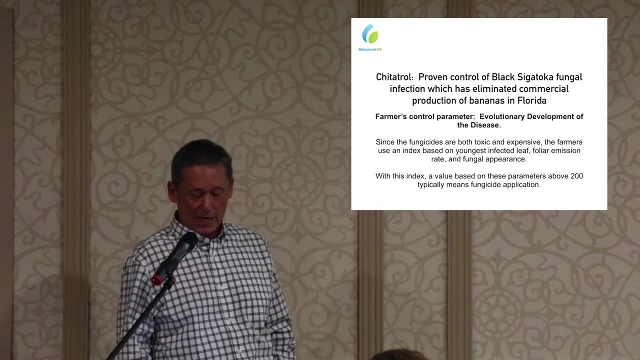 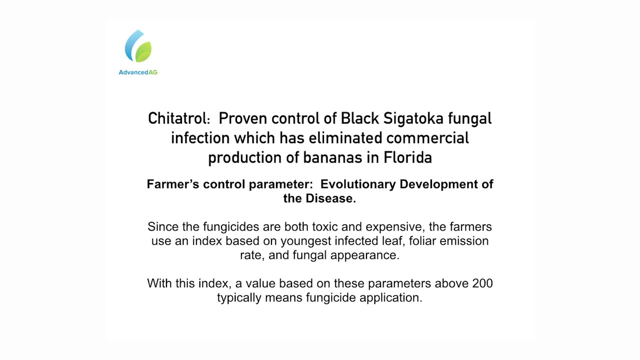 And by disrupting that cell wall you can attack a fungal infection. A really interesting project That we're now equipped with the efficacy data so that we're starting now officially with the US EPA and its counterparts in Canada to get biopesticide registration for the chitotrol. 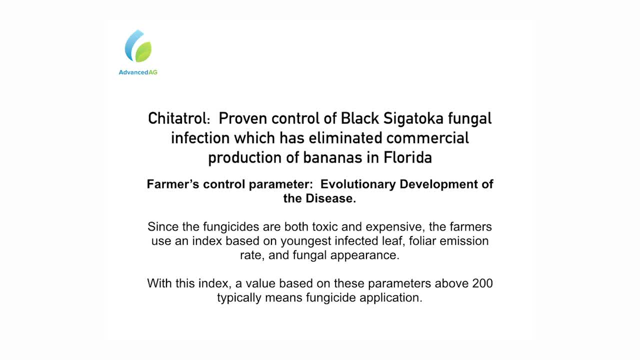 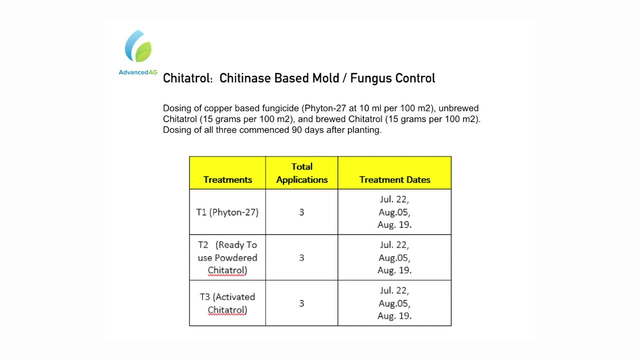 product. Black sigatoka is a fungal infection of bananas that literally stopped commercial production of bananas in Florida and is a real problem elsewhere. In a project in the Dominican which was run by one of their best agronomy schools, we compared the best. 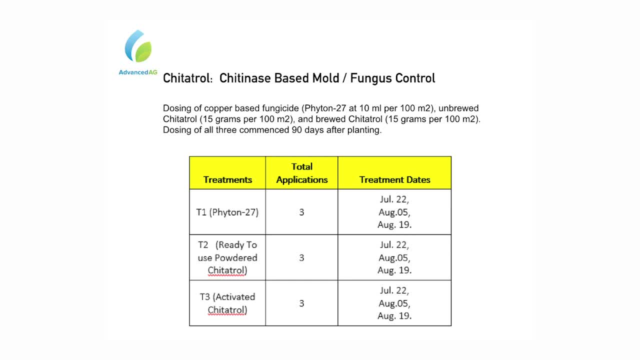 practice there, which is a copper-based fungicide, Phyton 27.. I think it's sold here in Canada: Chitotrol that's not brewed, that doesn't go through the tanks, and T3-activated chitotrol. 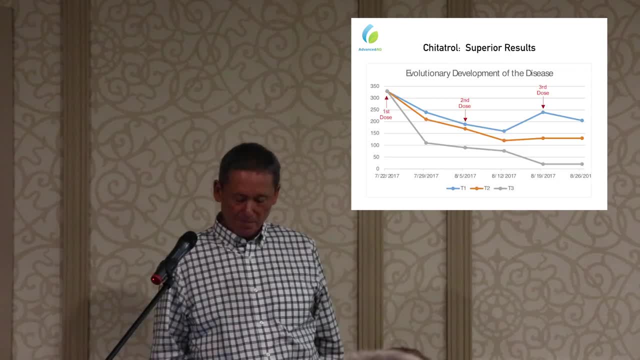 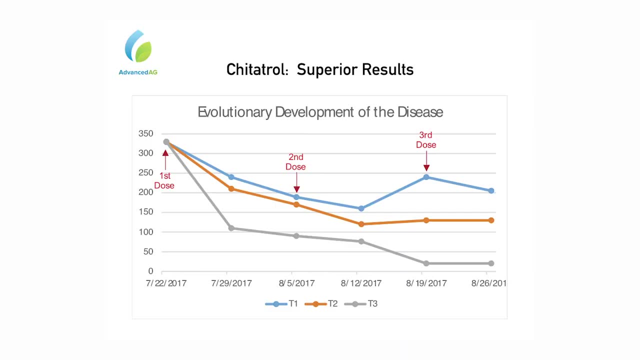 that means brewed. It goes through a brew process And what we have here is the standard practice has an index called the evolutionary development of the disease and they look at leaf eruption rates and visual things. But an index of 200 means apply more fungicide right away. 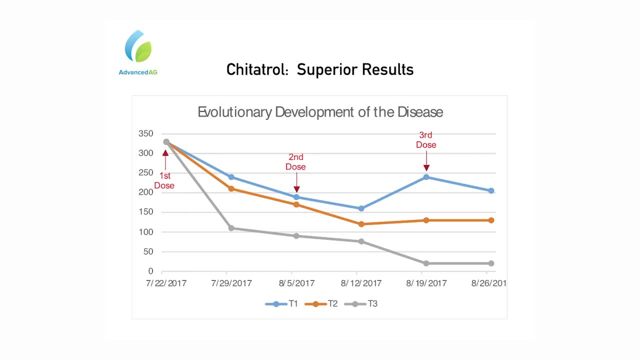 In this particular case this was started when all three control and the two chitotrol tests were started, when the disease was pretty severe After one dose. you see the blue is the Phyton 27.. It never really gained significant traction. 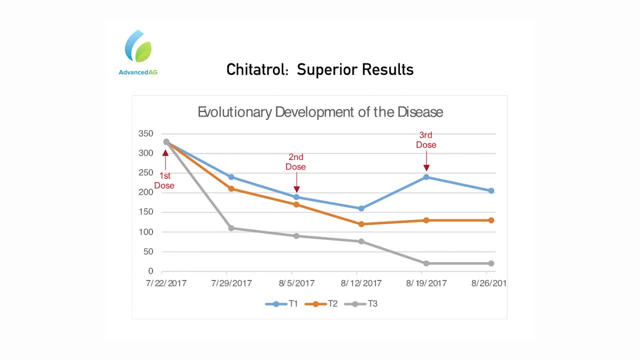 And again we started- or the researchers started- with a pretty high infection As we went there. the unbrewed powdered chitotrol did a decent job. It took a few days but it was a pretty good test, took it below the threshold for applying fungicide and the brewed chytotrol, which 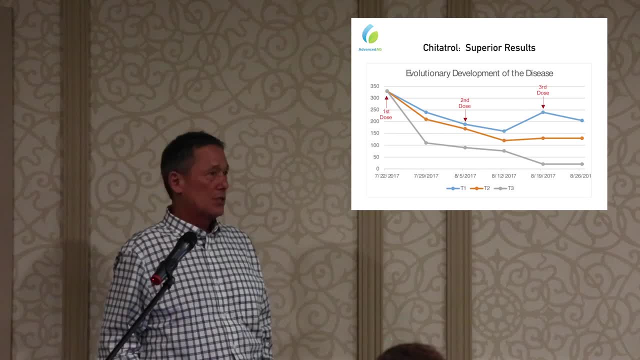 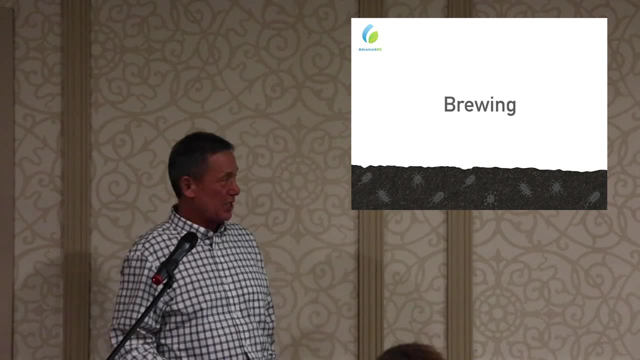 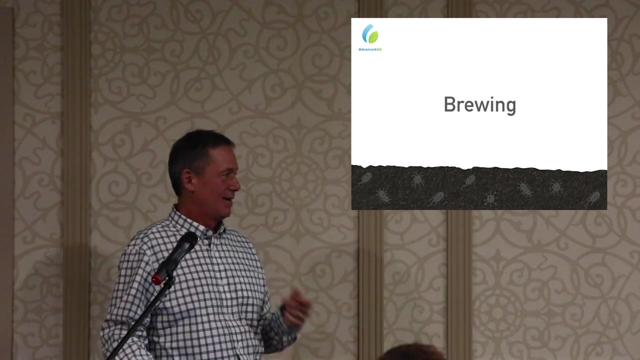 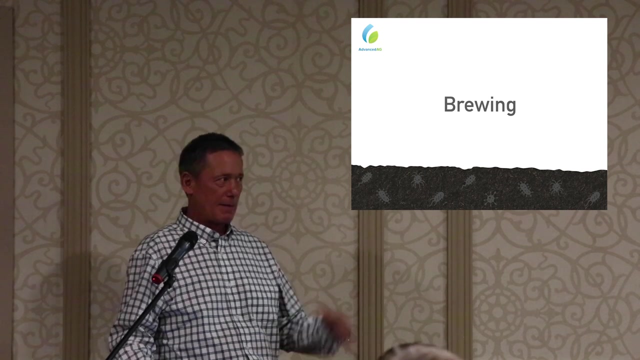 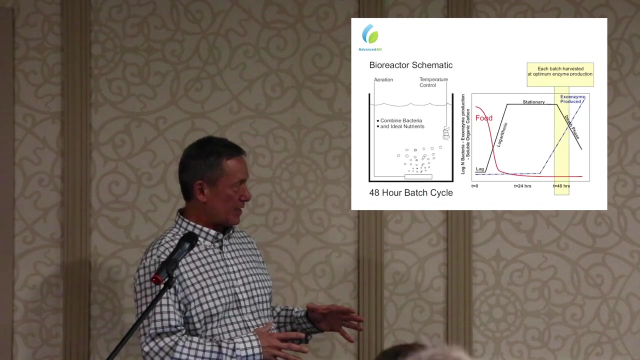 will explain. the tanks did a fantastic job. so the big thing: there is brewing and fortunately back in the States we like to do things sloppy and dirty. we don't have whatever the ingenuity to set up good brew stations. we just make bacteria perform functions or whatever. but the idea and we don't have to worry.